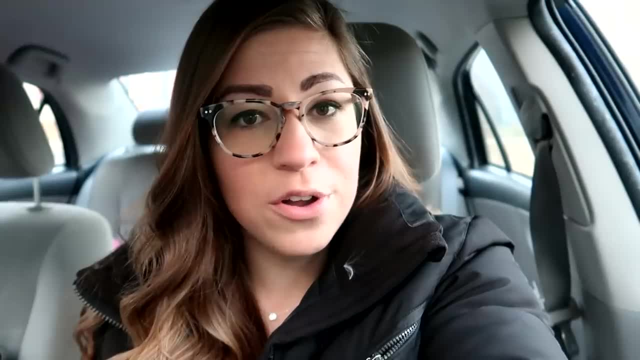 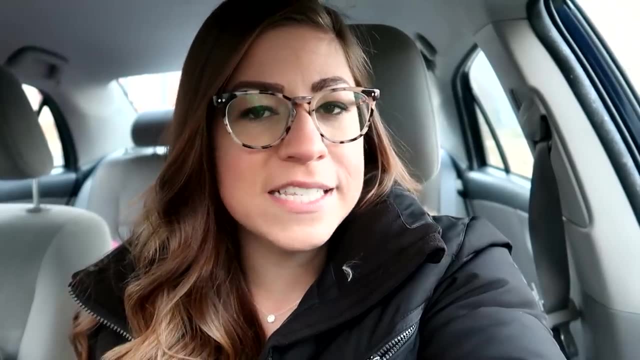 I am meeting with just one of my team teachers this morning because we are going on the field trip together and that's next week. We have to plan out some things because this field trip is a little bit different than normal field trips. It's one that's required by the 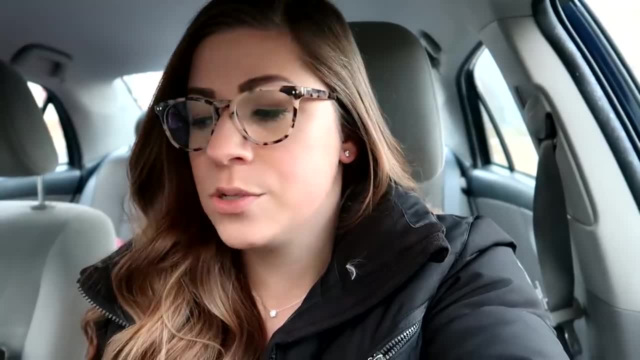 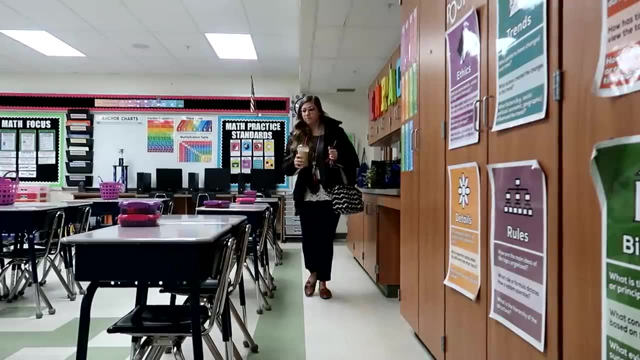 county for fourth graders and there's a lot of work that goes along with it. We're going to get that done and then I will catch up with you, probably during my planning time. I wanted to talk to you all quickly about my classroom doorbell, which I know some of you 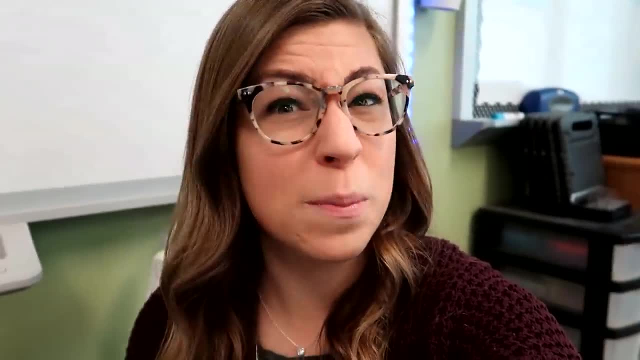 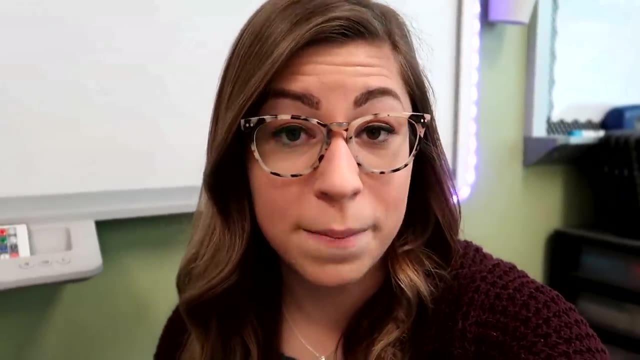 are familiar with, but I still get a lot of questions in terms of how the doorbell works and then how I use it in my classroom. and it works out perfectly, because I have a giveaway for you all. Quickly, in terms of the actual doorbell, the one that I use is from Sato Tech. 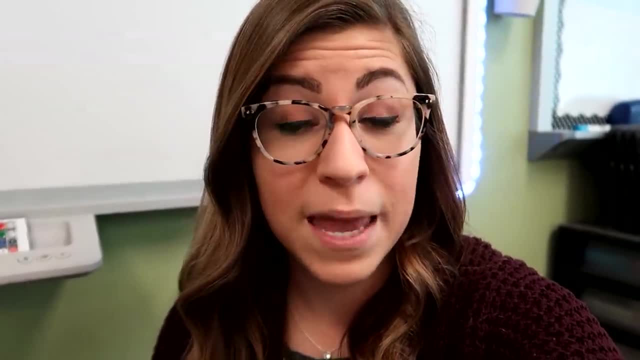 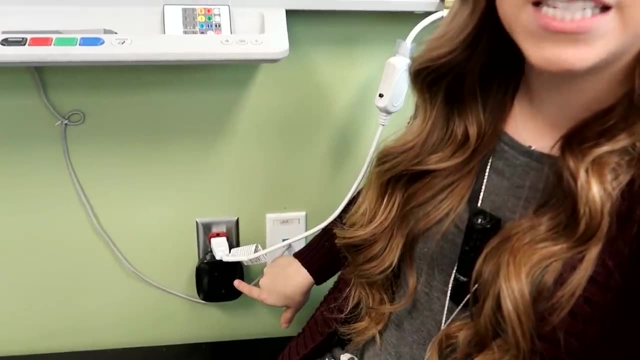 I'm down in the description box so you can check them out. You can get them directly from Amazon, Super, super affordable. It comes with two pieces. First is the actual receiver. This gets plugged into the wall somewhere in your classroom. Now I have mine plugged in, right. 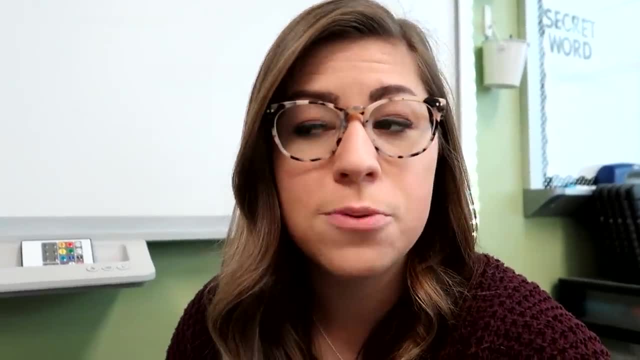 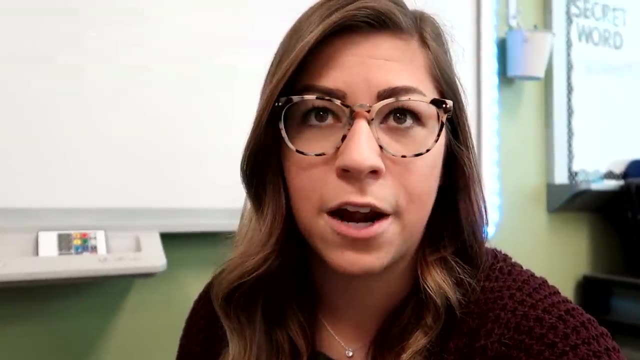 under your smart board, but you could plug it in anywhere around your classroom. I love that it plugs in instead of running off of batteries, so I don't have to worry about changing those ever so often. I feel like batteries, I just run out of them super often. Then there's also 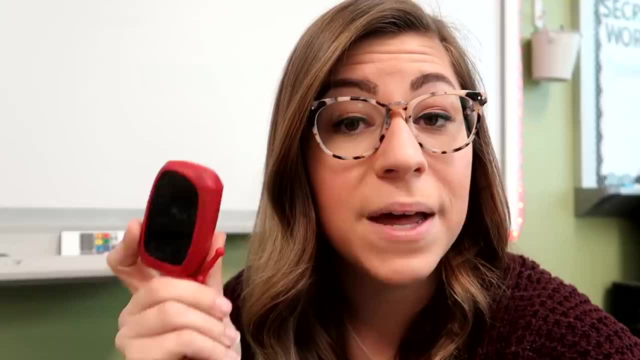 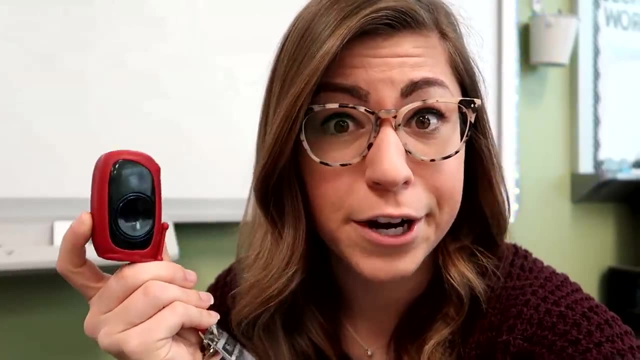 the button. Now, this piece is the button that I use to plug in my classroom doorbell and I unattached but I hang mine on my lanyard using a hand sanitizer holder. I got this hand sanitizer holder from TJ Maxx for a dollar. It's super, super affordable and the doorbell fits inside. 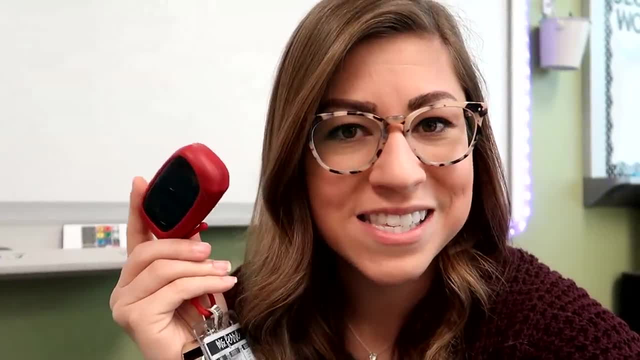 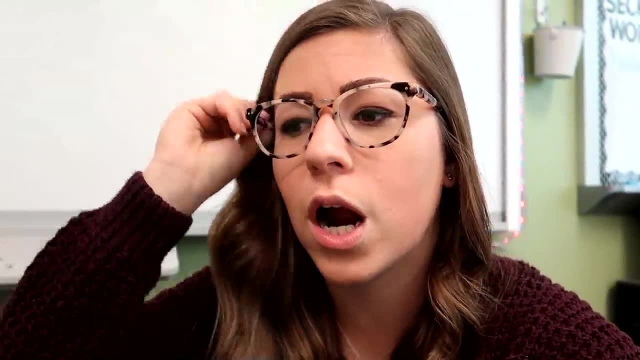 perfectly, and then I just hook it onto my lanyard. This piece does not come with the doorbell. The black piece does, The red piece does not. but you could also Velcro it somewhere in your room, or I know some teachers that have Velcroed it to their lanyard instead of using 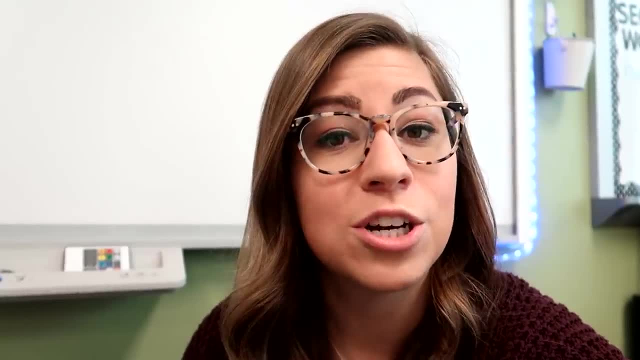 the hand sanitizer holder, but it's totally up to you Now in terms of how I use it in my classroom. I use it to get my students' attention, So if I click the button, the doorbell rings Now. 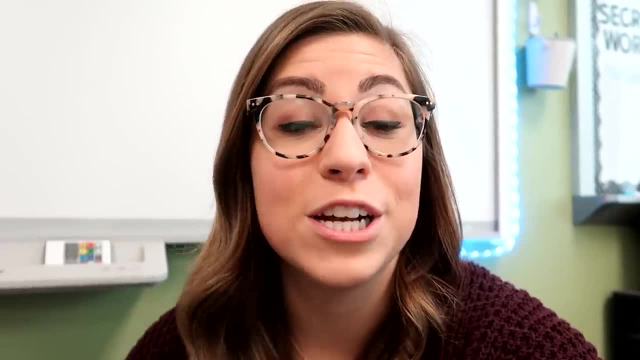 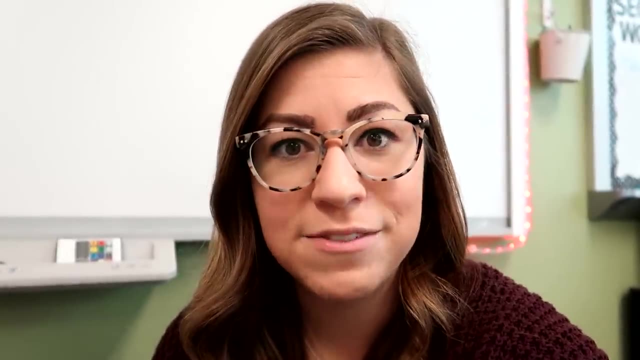 something else that I love about these doorbells is they have tons of different tunes, So as soon as your students start to get used to it and they're not responding as well, you can change up the tune. I also love they have different ones that are kind of like holiday sounding. I need to. 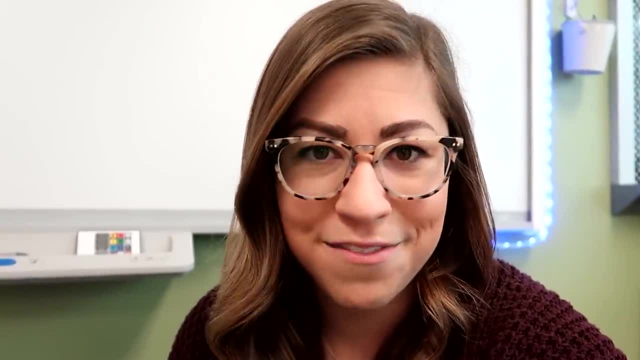 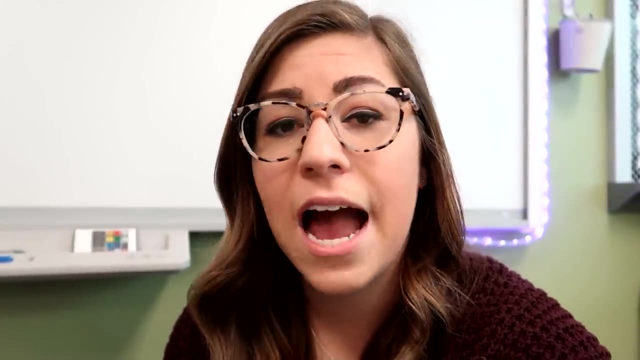 change mine actually to one of those pretty soon, but I love that aspect of it. You also can change the volume, so you can have it down low, You can have it up higher. What I just played for you is what I also love- and I know it's a lot of things I love. but seriously, this works from anywhere in. 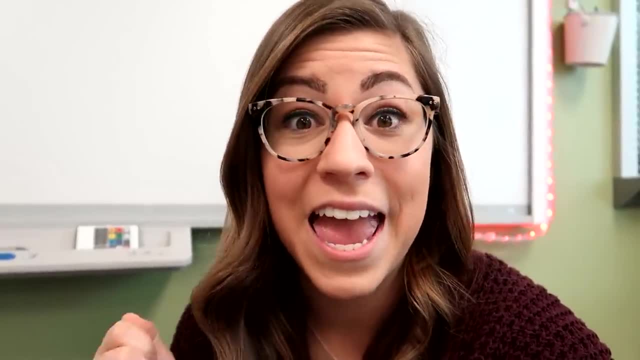 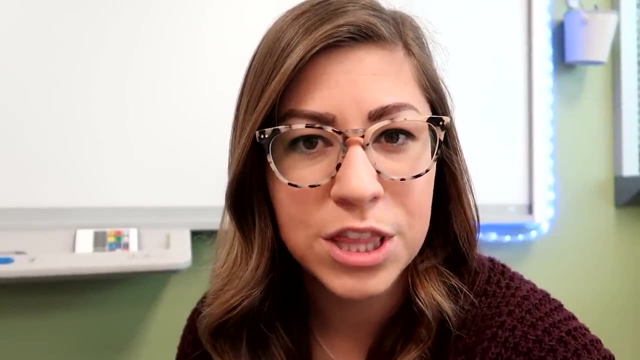 my classroom So I can be staying on the opposite side of the room and go ahead and click it and get my students' attention. Plus, because it takes a few seconds for the entire tune to play. sometimes I'm in the middle of having a conversation with a student and I'll go ahead and click it to start. 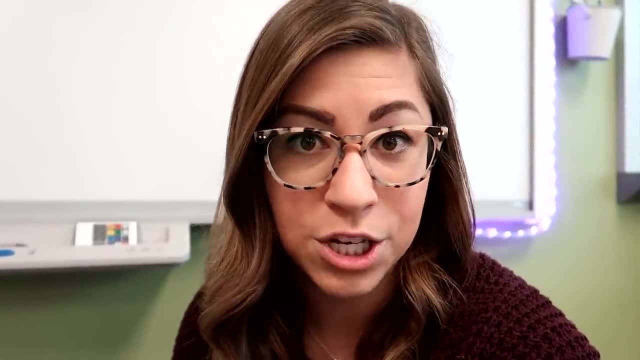 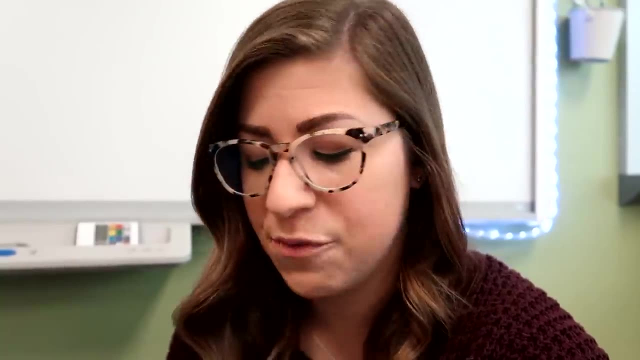 getting my other students' attention and by the time I finish that conversation, they're all ready to go. I also know of some teachers who use these in terms of switching between groups or rotations or centers. That's another option for you. I'm a little bit more of a fan of those. They're really cool. They're really really cool. 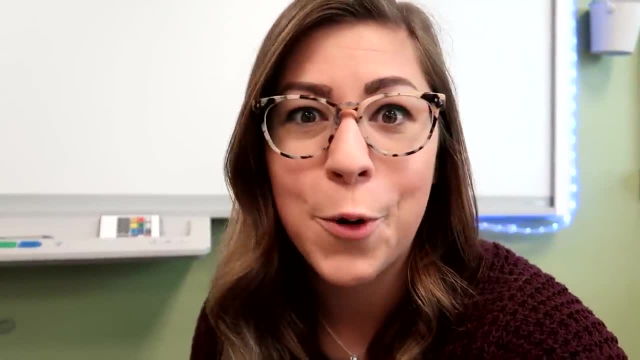 I've had a few students that have sent me some to give away. They had contacted me and they're like: hey, we'd love to send you one. I'm like I already have one. I bought it myself a year and a half ago. 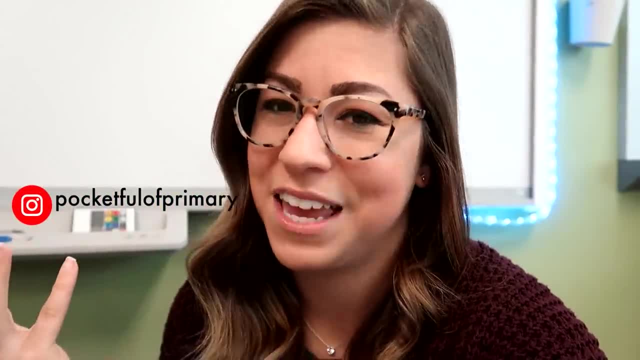 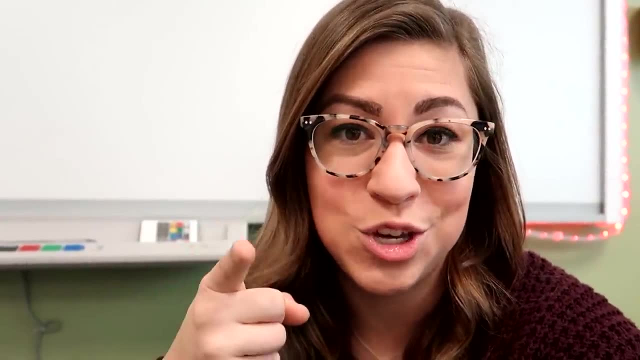 because I love them. I asked them if they would be willing to send some for me to give away. They sent me five of them. I've already given away two on my Instagram, which, if you're not following me on Instagram, you need to do that because I do some cool stuff on there. but that still leaves me. 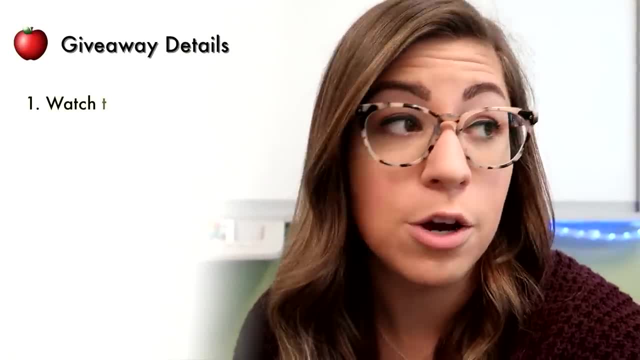 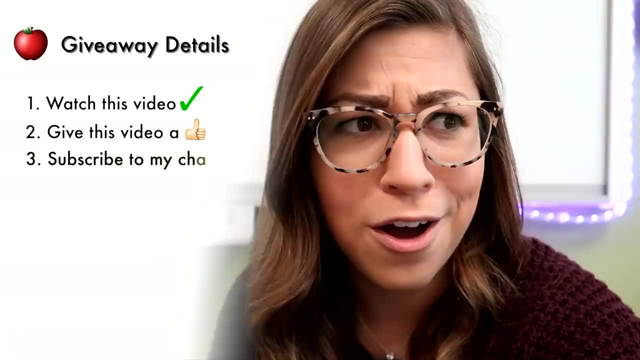 with three of them to give away to you all. Here are the details for entering the giveaway. I'm making it super simple. go ahead and give the video a thumbs up. number three: subscribe to my channel if you're not already, which come on, you should be. and then number four- I hate myself sometimes. number four: 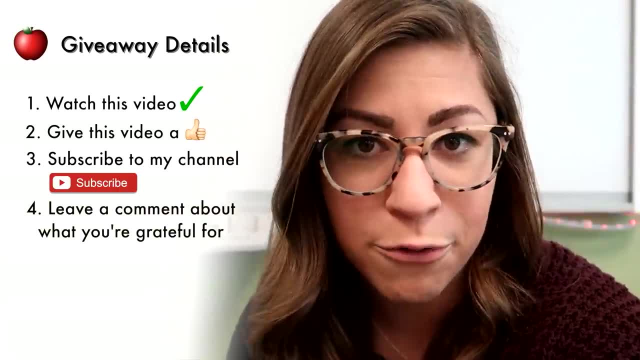 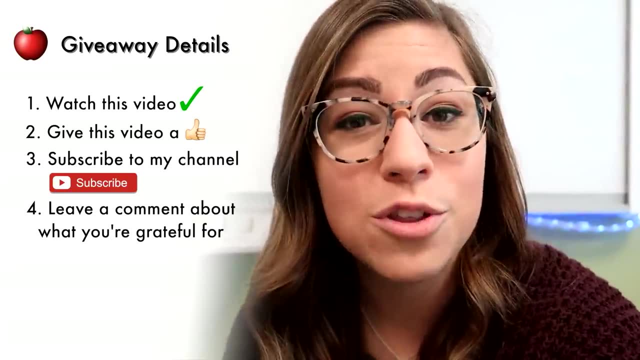 go ahead and leave a comment down below. I want to know something you are grateful for. I personally think that being grateful is highly important, and I love to hear what other people are grateful for. so go ahead and do those quick four steps. just watch this video. give the video a thumbs up. 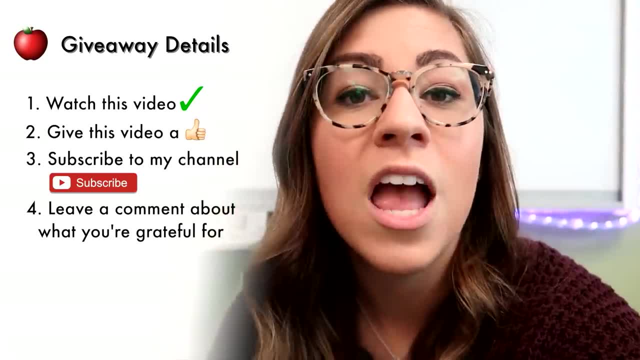 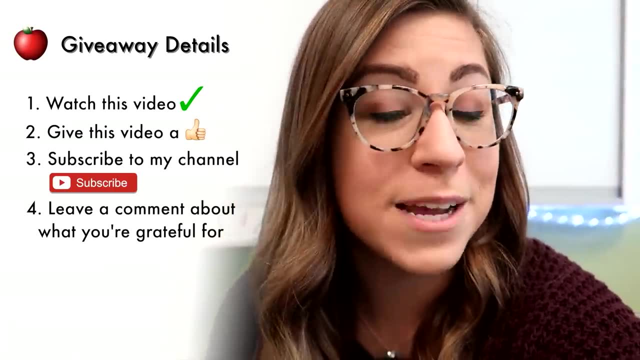 subscribe to my channel and leave a comment down below with something you are grateful for, you will be entered in that giveaway. I will respond to the three winners to let them know that they have won, and then I will get all the further information from you and I will send the. 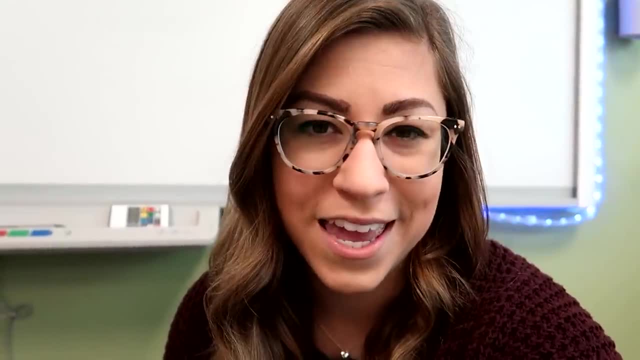 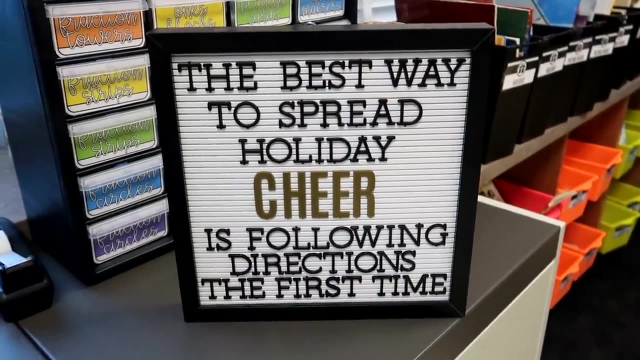 doorbells your way. I do have different color options available, but you may not get the specific color that you want, but still, it's a free doorbell and it doesn't get better than that. so I changed up my letter board for the holidays. now, this is not my original idea. I saw this all. 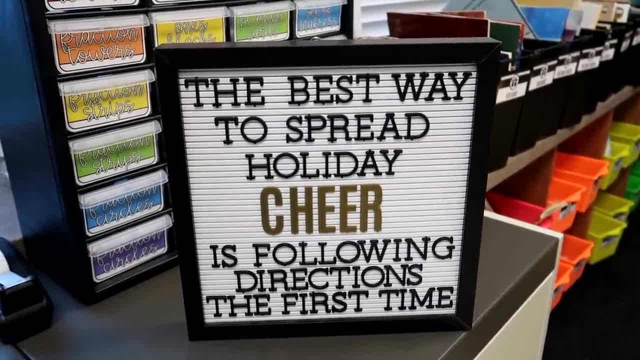 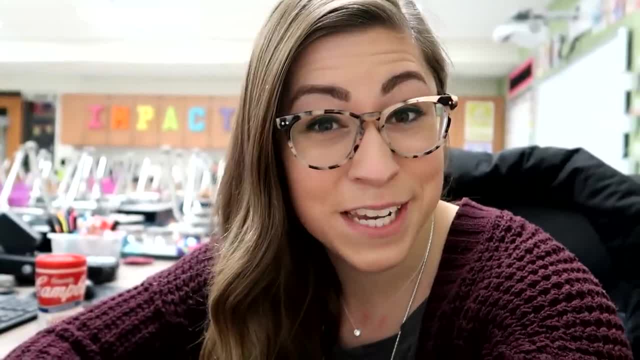 over the internet and decided to hop on the bandwagon. but it says the best way to spread holiday cheer is following directions the first time, and nothing has been more real than this statement right now, life of day. first of all, this kimball soup, not brand placement. I wish it was brand. 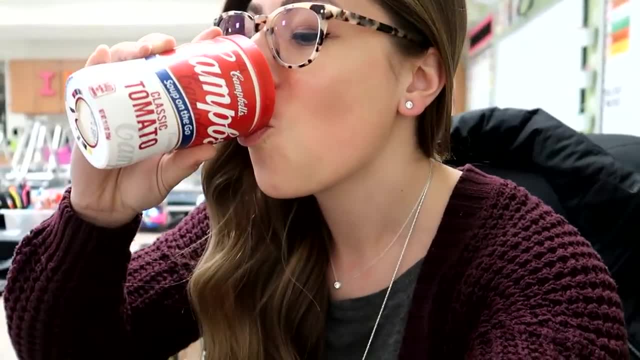 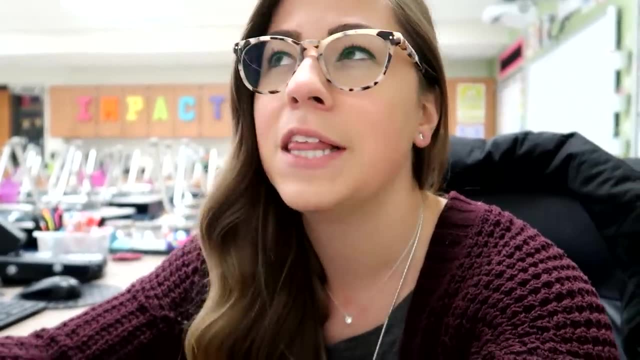 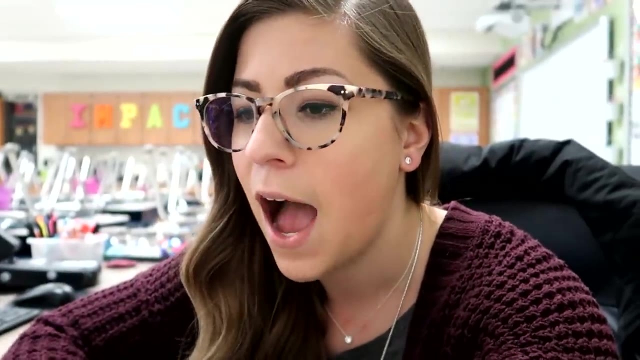 placement. I just drink this every day for lunch, but all right, so it is. what even time is it? it is almost six o'clock. I just feel like I'm living my best life right now. I mean, okay, in reality I just spent the past like two hours grading, so probably not my best life, but I feel so genuinely happy and 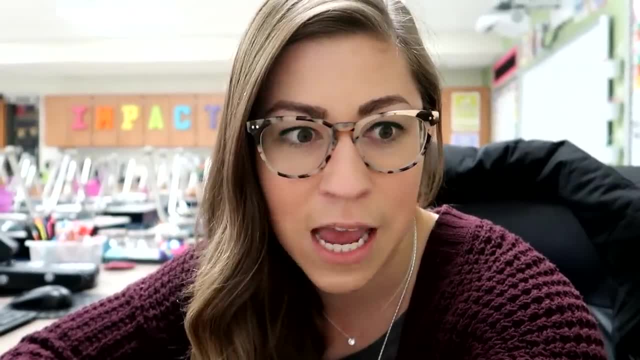 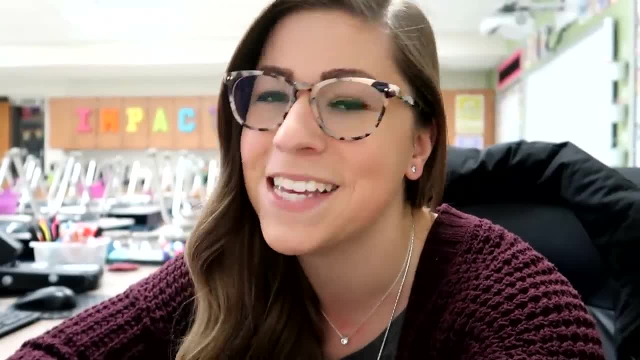 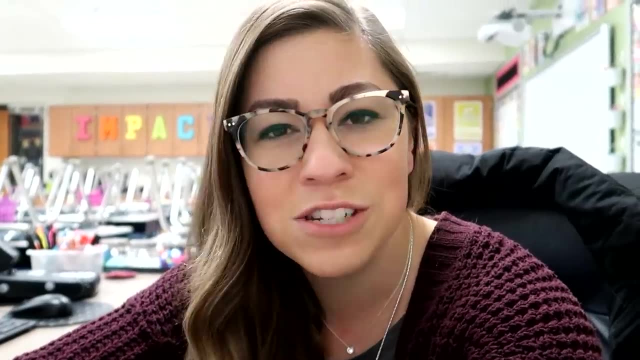 that was graded and I got a really good score. so I'm really happy about that, because I am totally a nerd and really care about my grades. I probably shouldn't, but I do. I'm a little bit of a perfectionist, if you haven't figured that out yet- but I also just am genuinely happy. I feel like 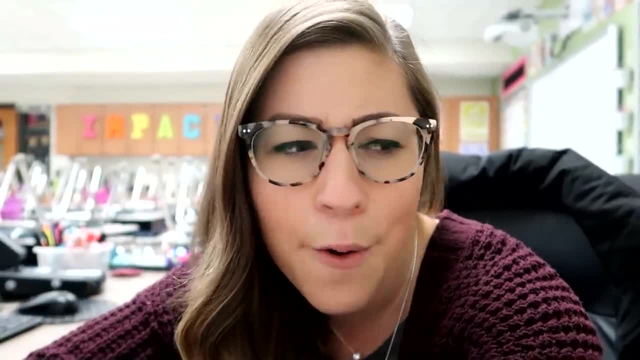 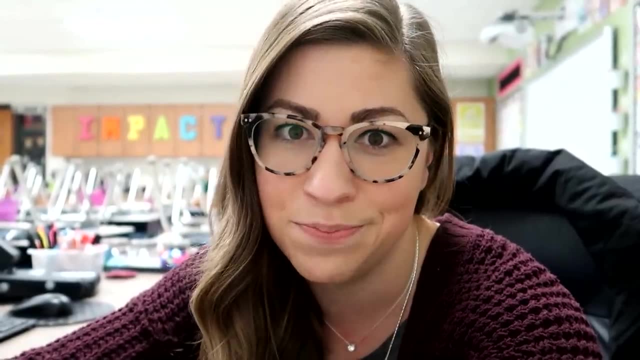 my day went really well and just the connections with my kiddos and all that good stuff. we had our funeral for Pluto and I know some people told me like well, maybe it's not actually dying. no, after seeing it today it- Pluto- is no longer with us. so we did have a little funeral and like half the grade. 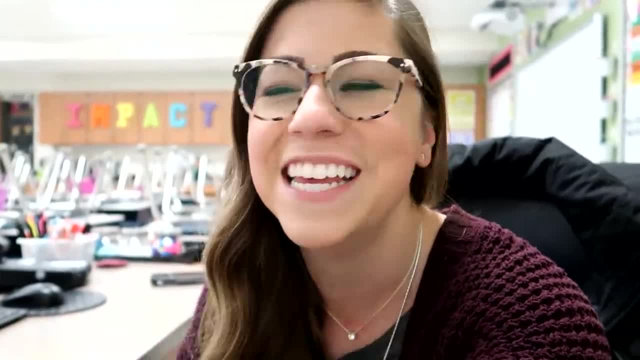 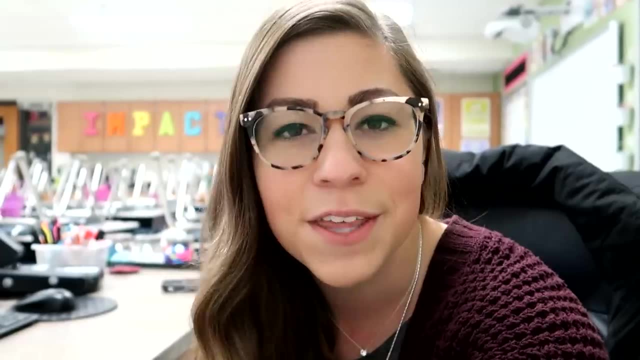 was swarmed around us, like all saying their good words, like Pluto was a great plant and we buried him outside. he will decompose and become one with nature again and I'm just, I'm just feeling good, I'm feeling really happy. so I need to get out of here. now that I'm done greeting, I'm gonna go to 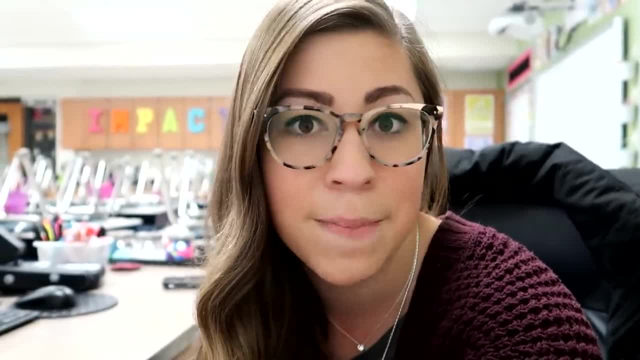 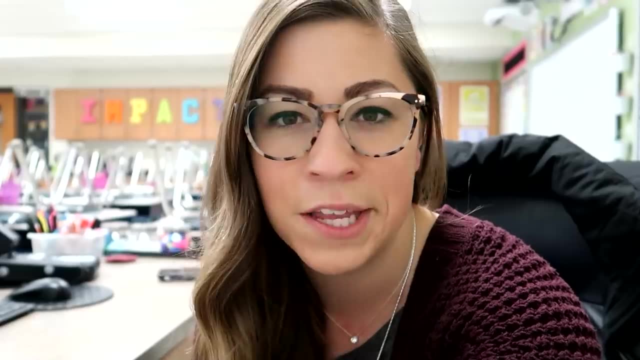 the gym, go home, figure out what I'm doing. tomorrow we are starting a metric measurement, so I'm excited and I like just starting something new, like we've been working on fractions for a while and like I'm over it, I'm ready to move on. so I'm saying so a lot. 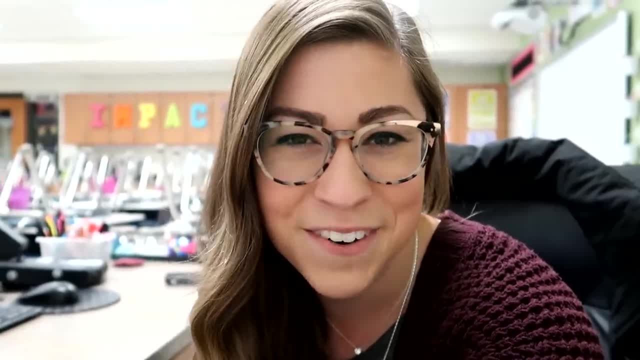 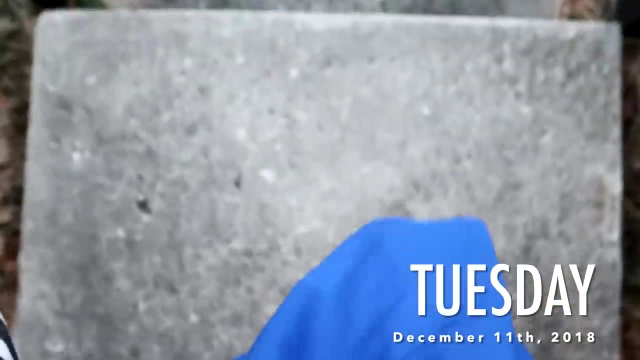 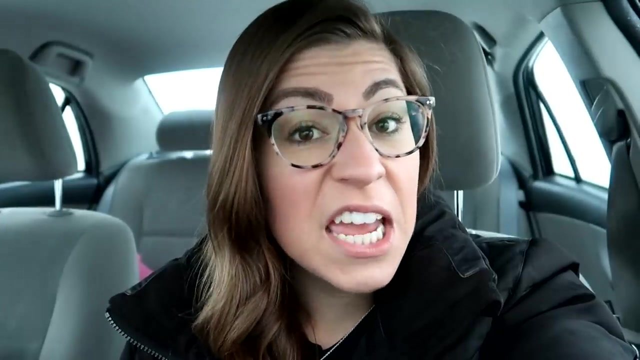 I apologize, I'm gonna get out of here. I will catch up with you in the morning, hopefully still in a good mood. good morning YouTube. I got excited this morning because Billy told me that there was a little dusting last night. that's not the reality. it is frost. and listen, frost is just. 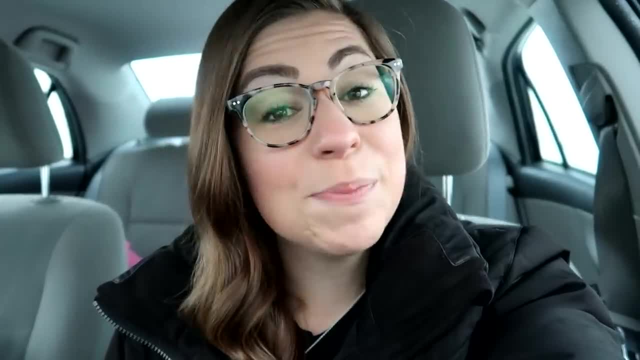 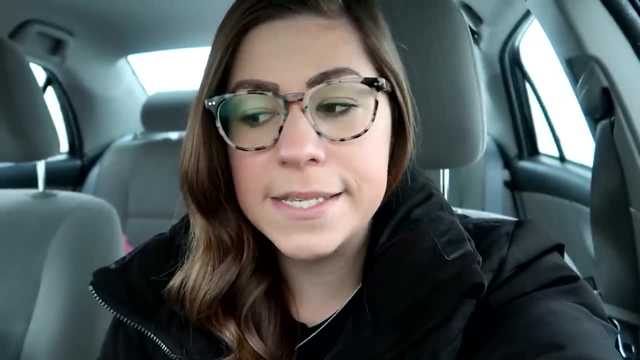 an inconvenience. there's nothing special about frost, so I was productive last night. I got a lot of things done that I needed to get done, one of which being I have to renew my certificate coming up, because in Maryland your teaching certificate is good for five years and believe it or not, I'm in my fifth year of teaching, so my certificate expires this summer. in order to renew your certificate, you have to get at least six professional development credits. I have already done that, which is awesome because most the time, your County provides you with opportunities to get. 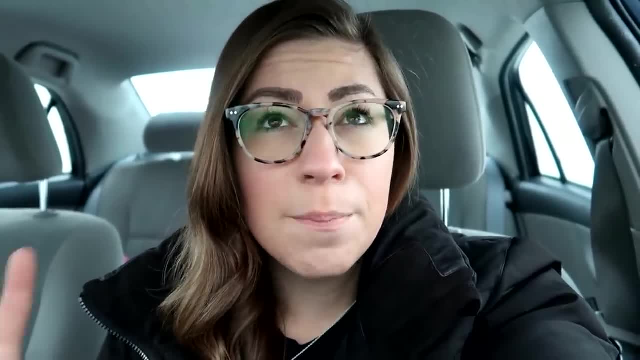 those and I've already completed them. but I did have to fill out a like professional development plan or something. but I had to fill it out with my information, list out the credits I've already done and then I have to get all my certificates done. so I'm gonna get ready to go out and do all the 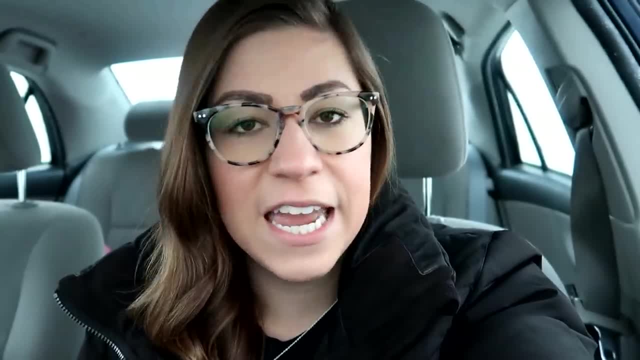 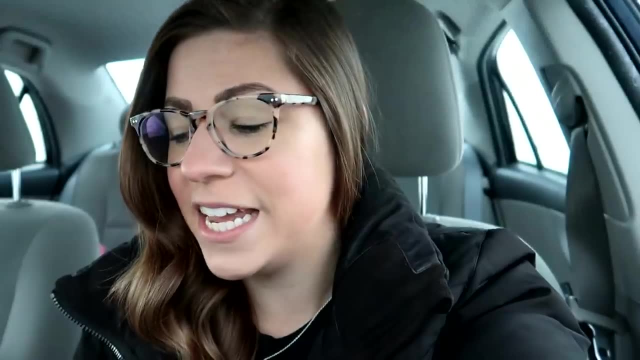 I had to sign it and get my administration to sign it, and then I had to scan it and send it to those people And then they will take care of getting my certificate renewed for me. So that is done. I'm excited about it. I also had to send some stuff, since I'm the e-coach and I do professional development after the professional development. 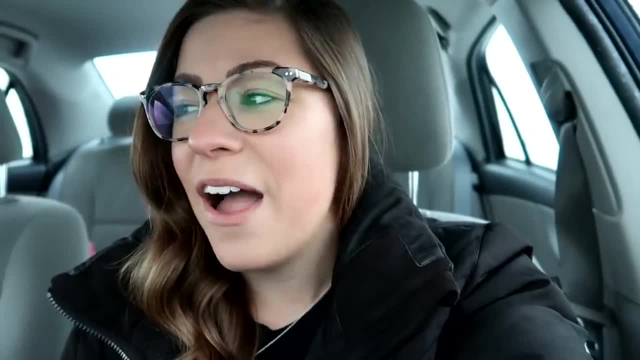 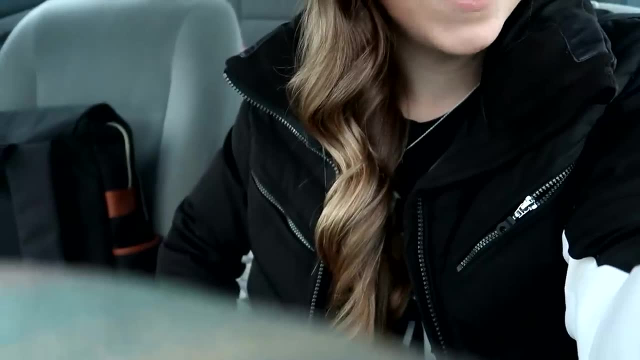 I have to send a signed copy of the sign-in sheet. So I feel good. You know, I got those like little things done that I needed to get done and I made a deal with myself that if I do my Hair in the morning, hair is done, I get to go get coffee, and so far. 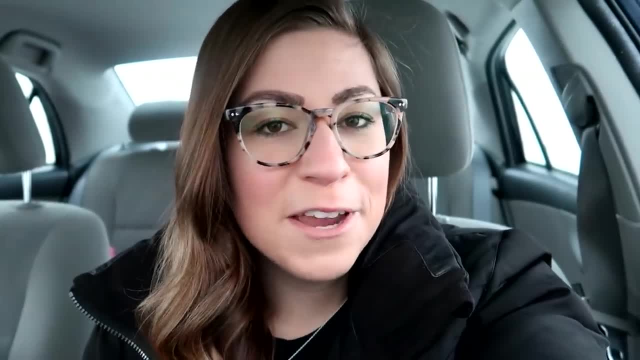 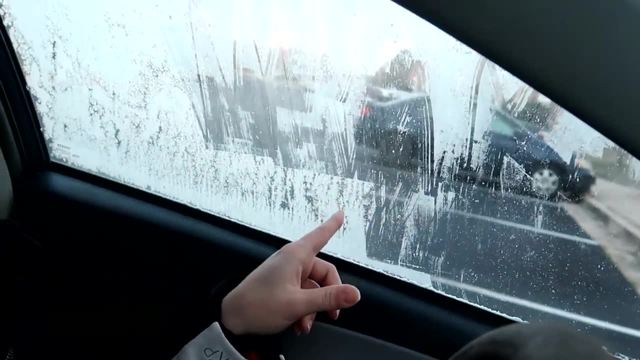 It's really motivating me. so because I just froze off my fingers trying to scrape my windows, which I'm a bad person. Let me just show you for a second. I just like carve a little hole. I do not sit there and scrape the entire window. 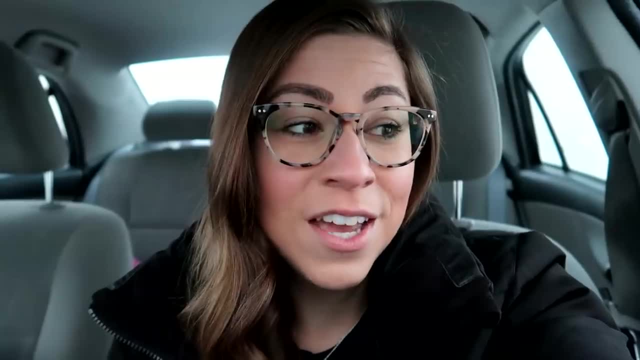 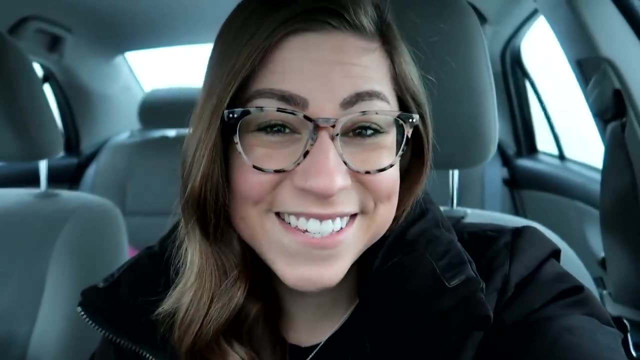 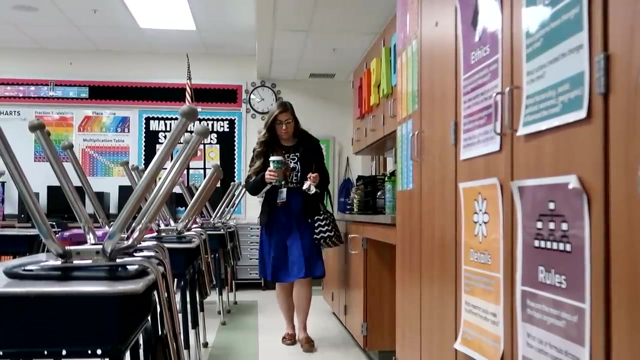 So for those of you who think I'm a good person, think again. I only do the least about possible when I am, you know, scraping off my window, But I'm gonna go get myself some coffee as a reward and then we get to school. I Wanted to do a little outfit of the day and, you know, maybe one of these days 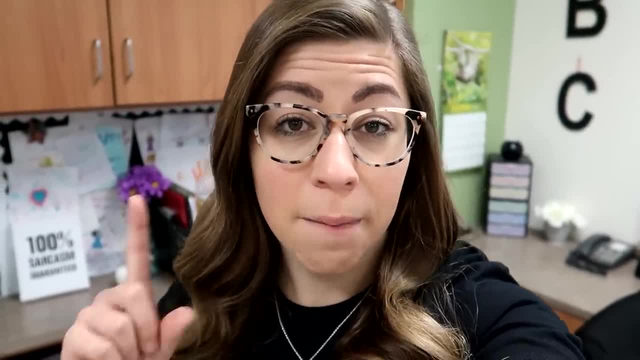 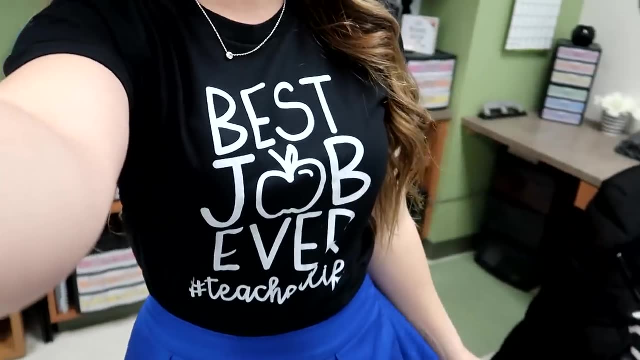 I will get a full-length mirror where I can do these properly, but that day is not today. So the main reason is because I want to show you my shirt, because it's adorable and it just came in the mail yesterday. It says a best job ever. hashtag: teacher life and the O in job is an apple. 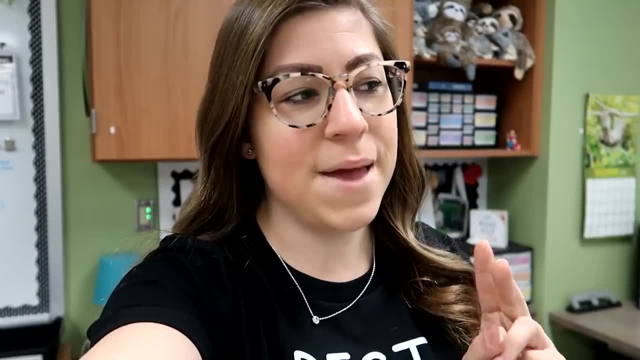 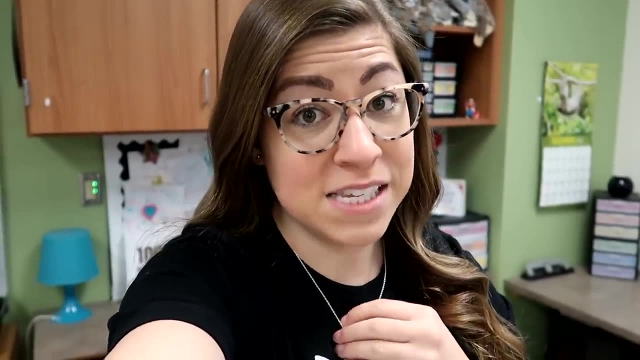 Good news, bad news. good news: This shirt is absolutely adorable. bad news: I don't think I can really link it. I got it from Jane comm, which, if you're not using Jane comm, first of all, If you're anything like me and you buy stuff easily, you probably shouldn't use it. But you know, if you have some self-control. 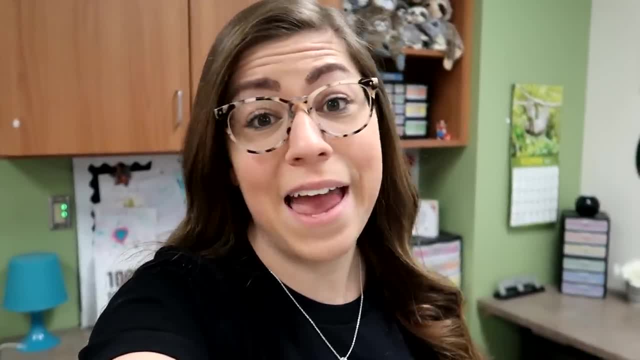 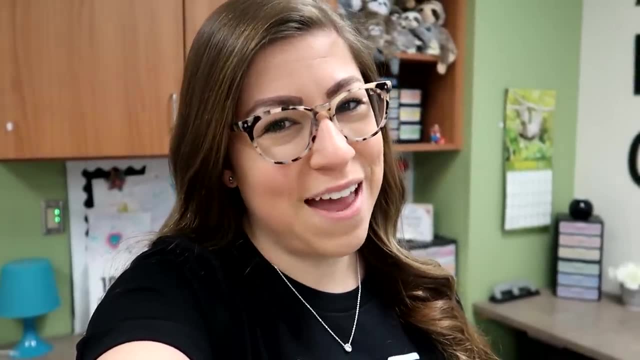 It's an excellent website. They always have deals and it's a lot of like small sellers and I just love it. Now, that being said, the deals run out and once the deal runs out, unless you can track down the website, You don't really have a way to link it, and I tried to track down the website last night. 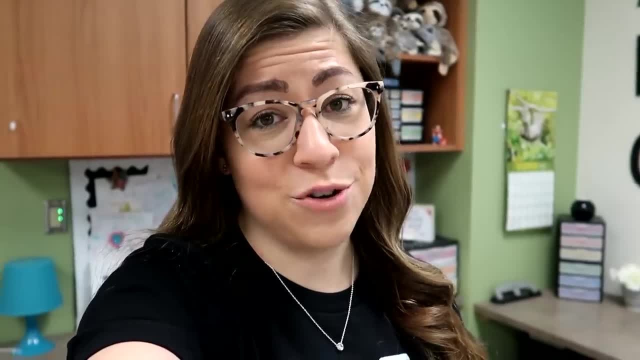 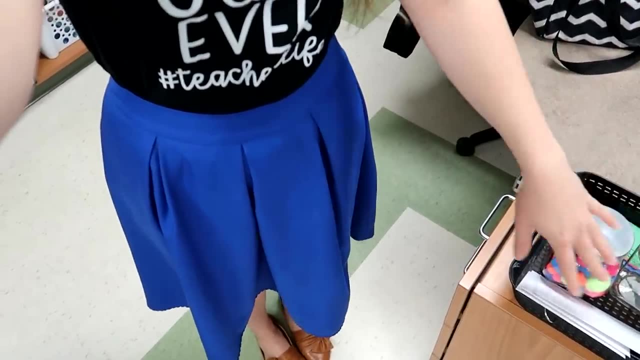 And I couldn't really find it. if I can, I will link it. if not, don't hate me. Then I have my blue skirt. I'm still getting asked about these skirts a lot. They come from Amazon. just ignore all of this mess over here, but they come from Amazon. They're super affordable. 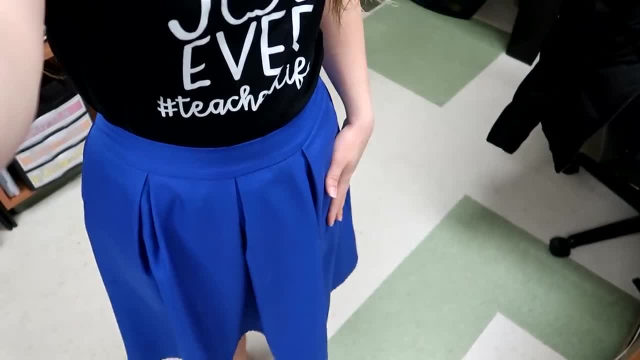 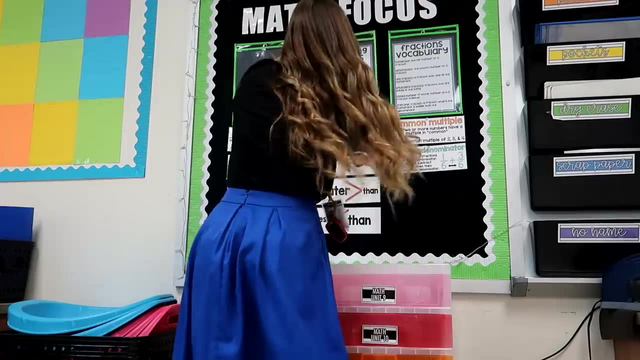 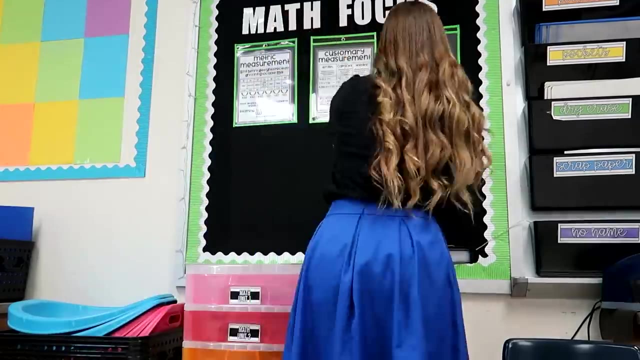 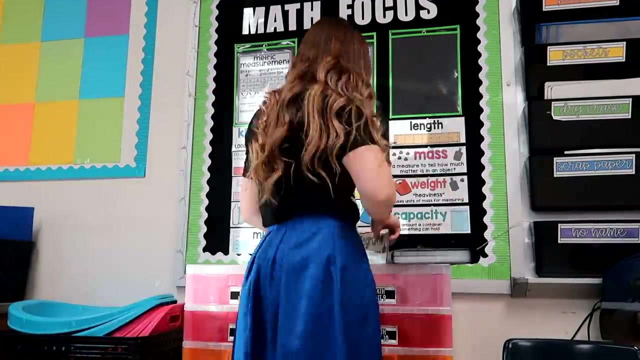 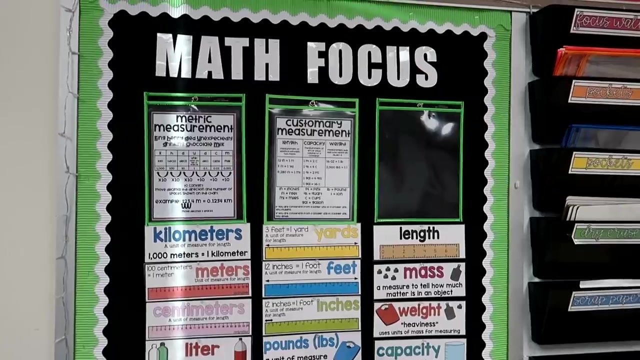 They're about $20 each and they have pockets, So I have this in like six different colors. highly, highly, highly recommend it. They are becoming more and more over the years in some areas. I just updated my math focus board. I do this every unit and we are starting a new unit today on. 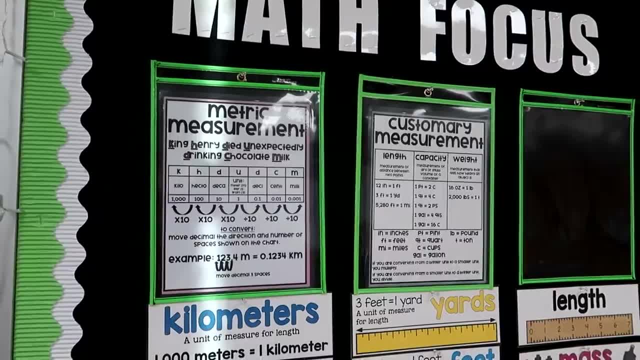 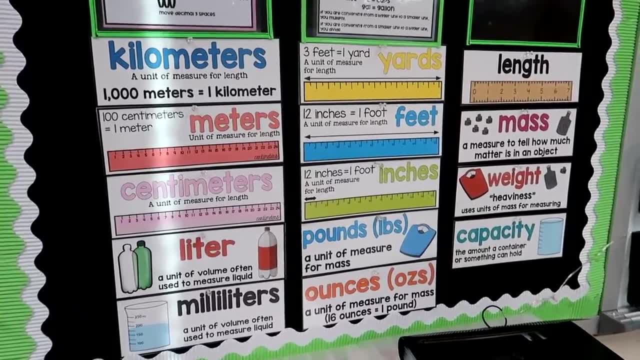 Measurement conversions, So we cover metric measurement and customary measurement. So first of all, these posters are from TPT. I want to say it's from math facts and backpacks, So I will link that in the description box. These vocabulary cards are talk about how I actually store these, because we have 15 math units So I have a lot of vocabulary. 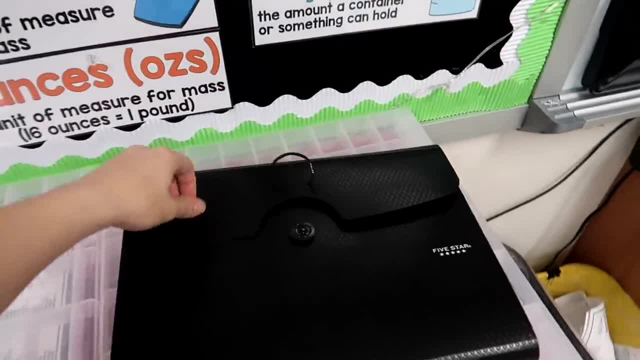 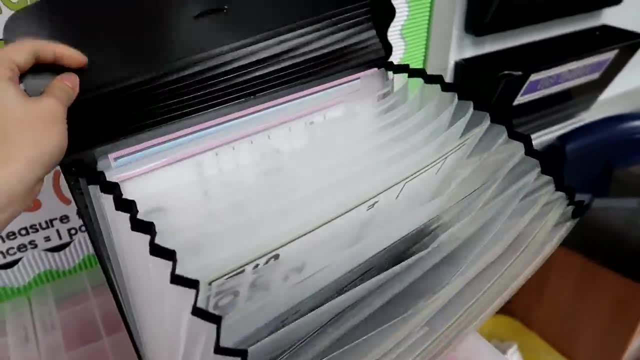 cards and a lot of posters. So I actually got this organizer from Target. So it's just by a five star and it opens up and it has these dividers. So each different divider represents a unit, Basically, when it's the start of a new unit, I just find the unit in here and I already have all of the. 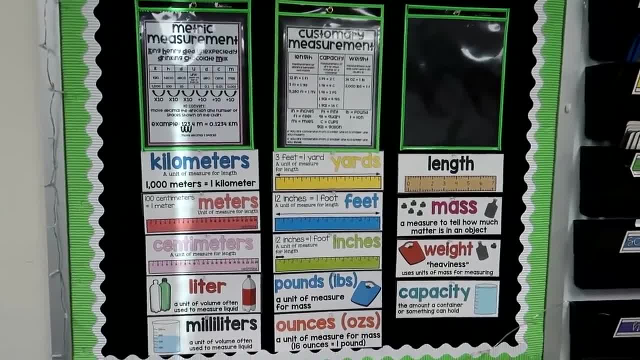 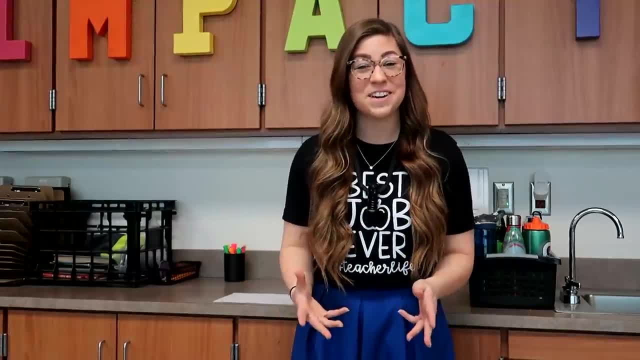 vocabulary cards and all of the posters that go with that unit. So it's super easy to just quickly change them out and then put them away and save them for next year. All right, I know this is a little bit of a different setup for me and I know I'm off center and it's probably bothering some of 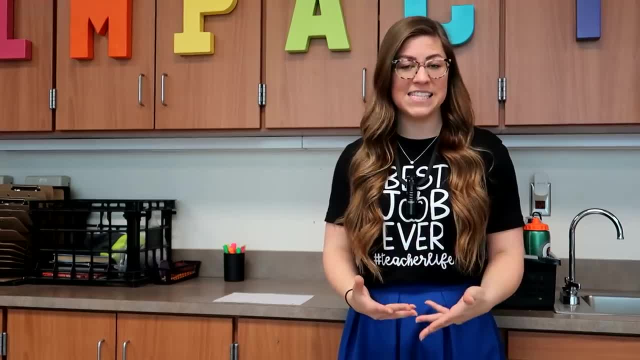 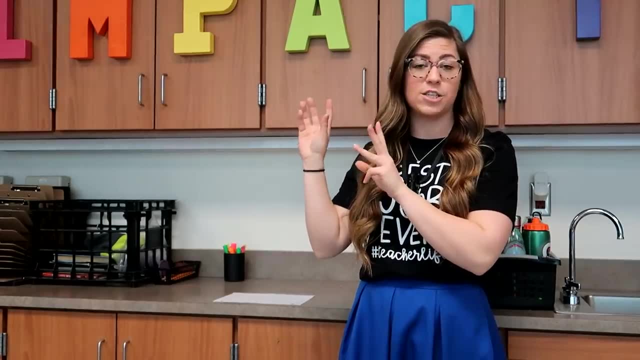 you It's bothering me, But what I'm going to do is talk through my lesson today and talk about how I'm making it more interactive for my students and working in more opportunities for movement. So I'm going to put up JPEGs on the screen of the slides that I use, because I teach every single day. 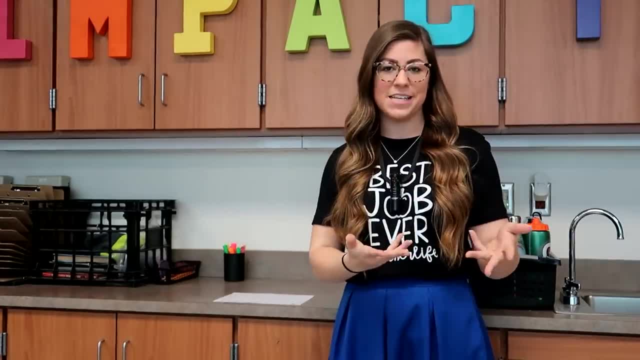 using Google Slides, So that way you can kind of see what the slide is and then I can explain what I'm doing. First of all, a little bit of background information, The way our curriculum is designed. we have three different types of lessons in math. 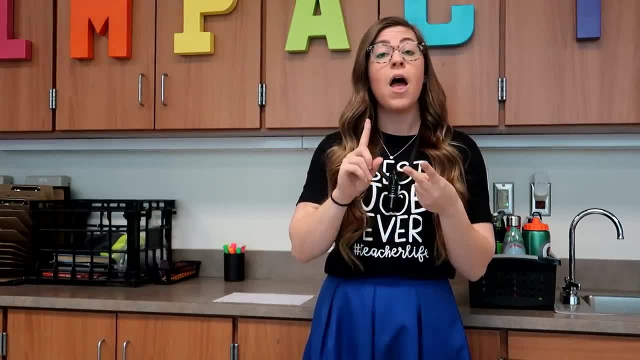 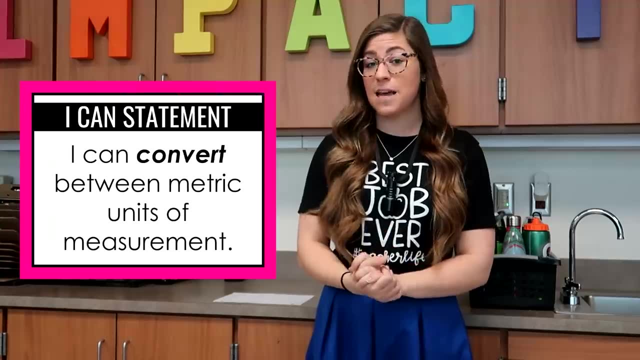 A conceptual lesson, which is when you're introducing a new skill, A fluency lesson, which is when you're practicing a skill, And then application, which is when you are applying the skill to a real life situation. Today is a conceptual lesson because we are starting a 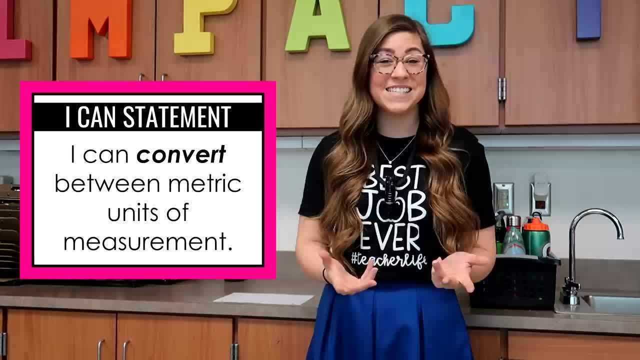 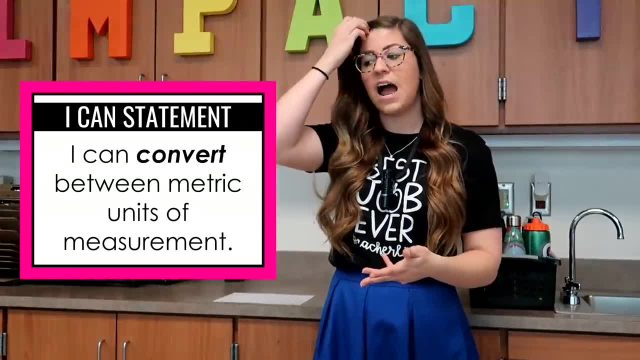 new unit And typically conceptual lessons are kind of on the boring side because it's new information And once you start practicing it with the fluency then you're able to incorporate more activities. But I've really been struggling with the conceptual lessons because the way 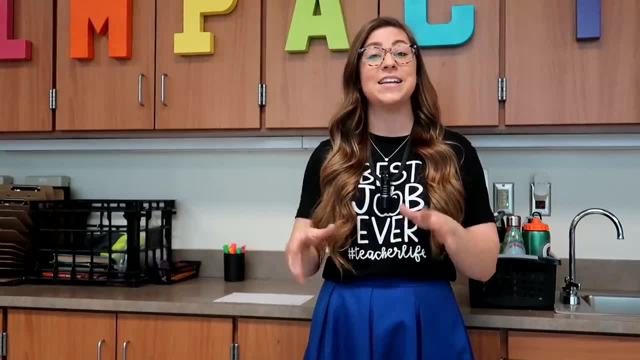 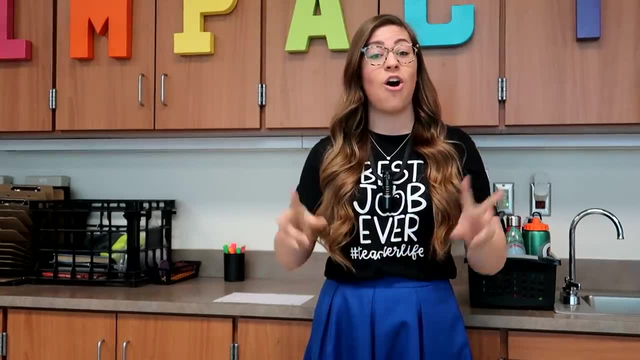 they're written into the curriculum, they're kind of boring. So I'm going to talk to you about how I take the curriculum and then make it work for me and my teaching style and my students. So our lessons always start off with what we call a number sense routine. This is basically a way to 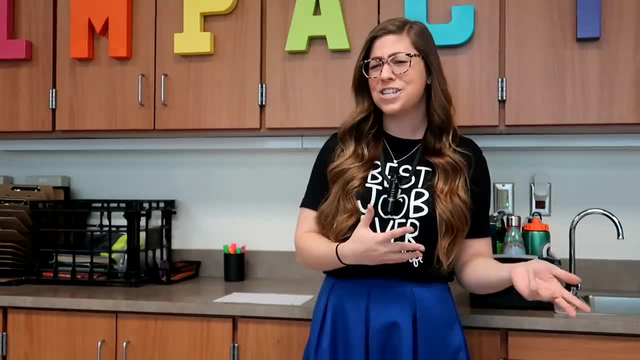 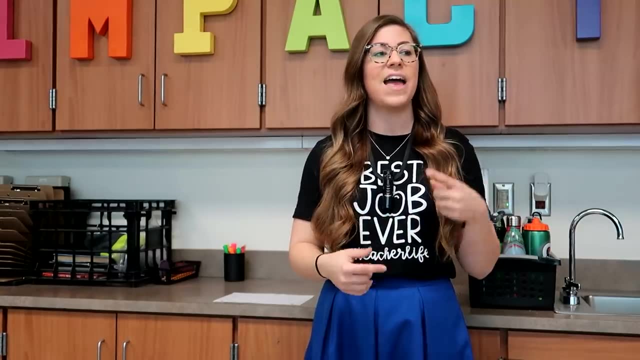 practice fact fluency. It's not always necessarily multiplication facts or division facts, but it has to do with whatever skill we are working on. So in the curriculum it wanted us to get into a circle and then skip, count around the circle, And I just knew that that was not going to work for me and I 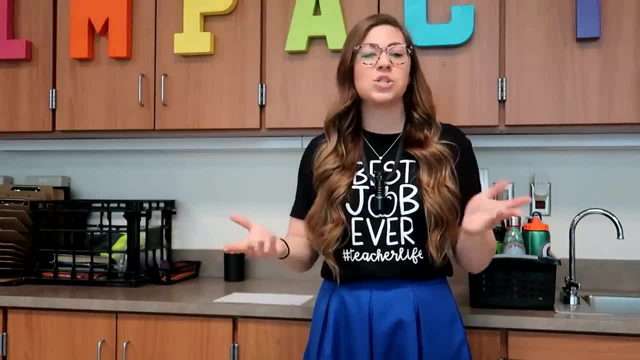 didn't want to get into a circle, And I just knew that that was not going to work for me. and I didn't want to get into a circle and just skip count, And it just wasn't going to work. So I'm doing something I call speed counting. All you need is a piece of paper. Oh, there go my notes. 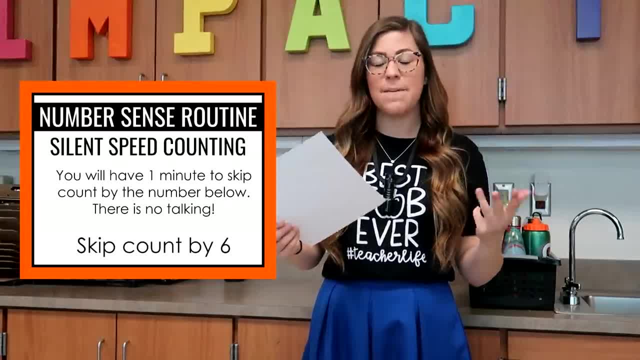 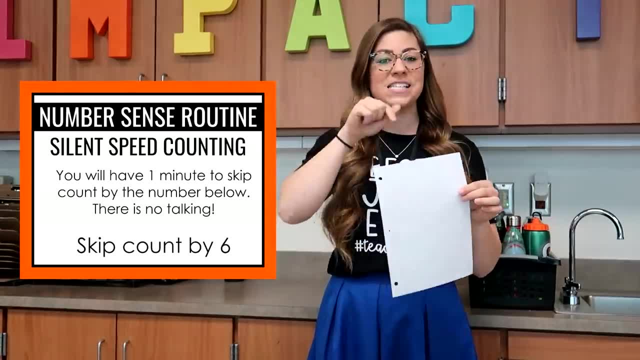 Okay, You can use line paper or you can use white paper, Doesn't matter. Essentially, students work in groups. I have my students work in groups of four and it's silent, So they're not allowed to talk and they pass the paper around and each person writes the next multiple. So if we're 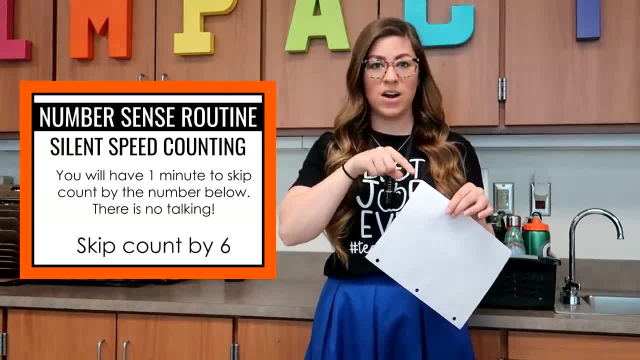 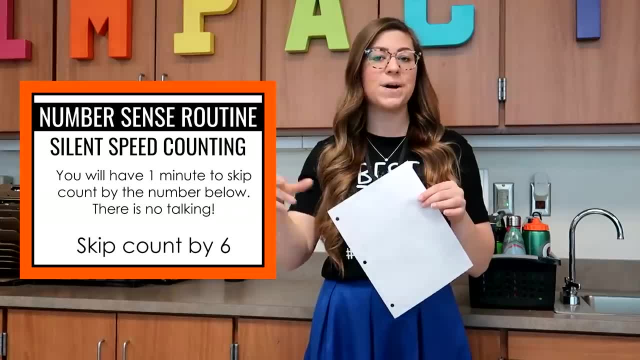 skip counting by sixes. the first person would write six, the next person would write 12, and so on. If a student disagrees, they can erase it and change it, but they cannot write another number. I time them, I put up a timer for a minute and we see who can get the most during that time. 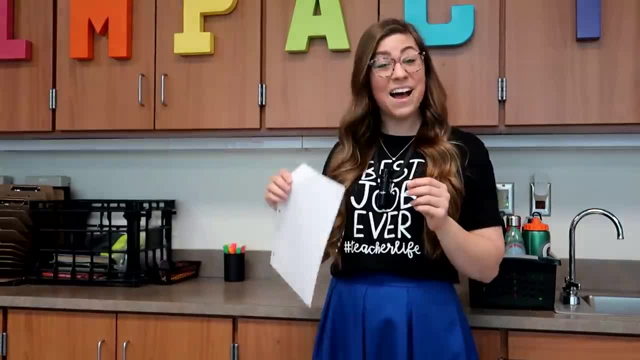 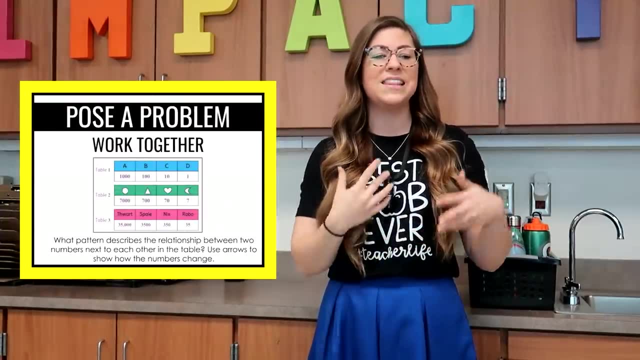 I don't usually reward them for it, but you could do that if you wanted to. After the number sense routine, we have what's called a pose a problem. It's typically a word problem and it's either meant to elicit prior knowledge or kind of introduce the skill and let them have a productive. 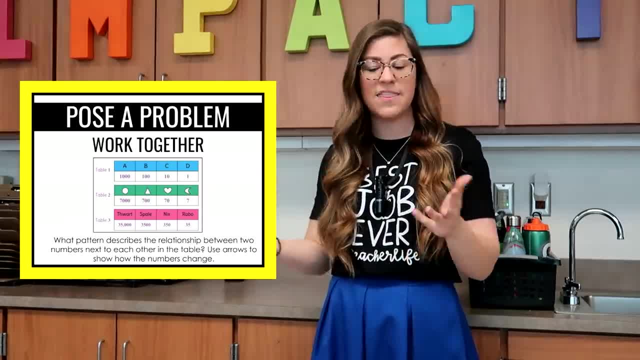 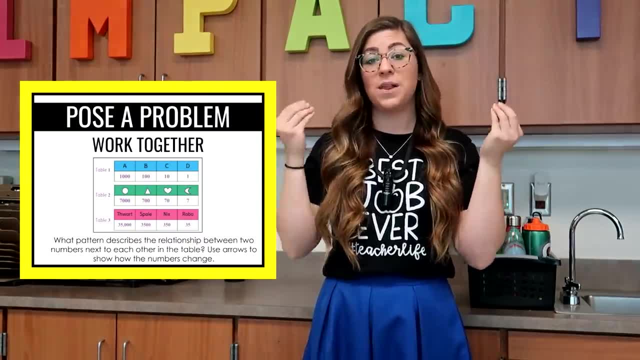 struggle to work through it with manipulatives and strategies and things like that. So this pose a problem- is actually liked because it introduces students to connecting metric measurement to place value, So seeing the connections of 10 times greater or 10 times less. So we're going to do. 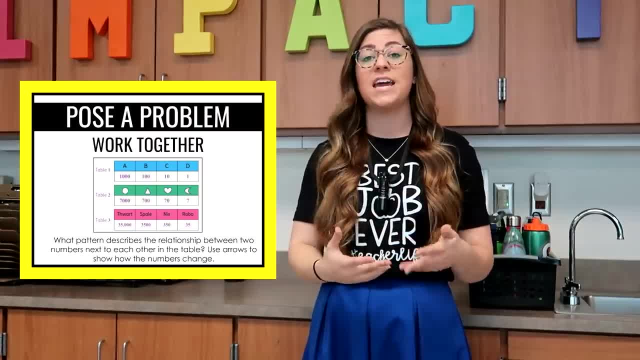 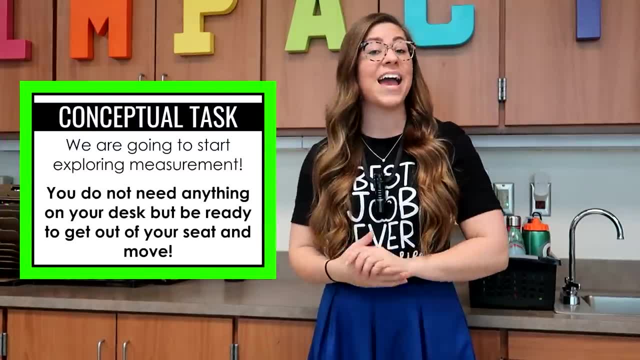 the pose a problem, as usual, They work together in groups and they solve it, And then we look at different strategies under the document camera, discuss it, all that good stuff. Then I'm actually going to show them a slide show. Now I got this off of TPT so I can't show the actual slides. 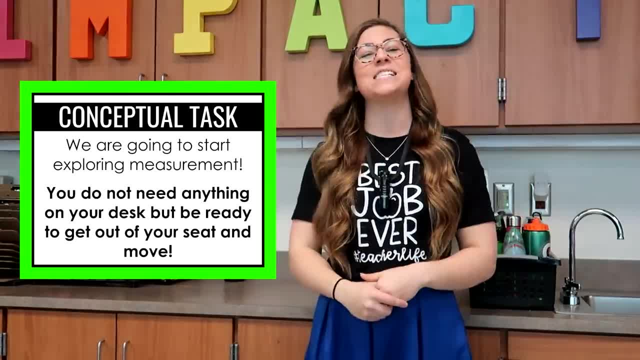 because I didn't make them, but I will link it for you in the description box. It's by Deb Hansen and she makes amazing slides, So I'm going to show you the slides. So I'm going to show you the slides. I'm going to show you the slides. So I'm going to show you the slides. I'm going to show you. 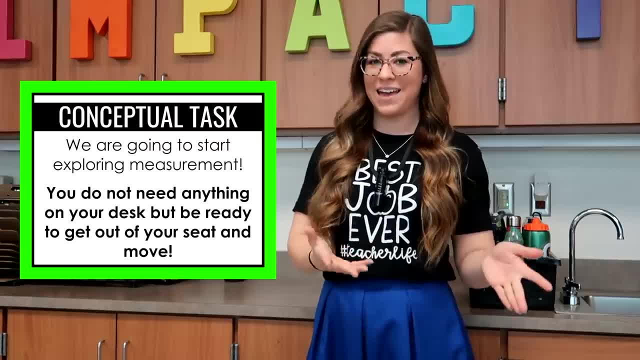 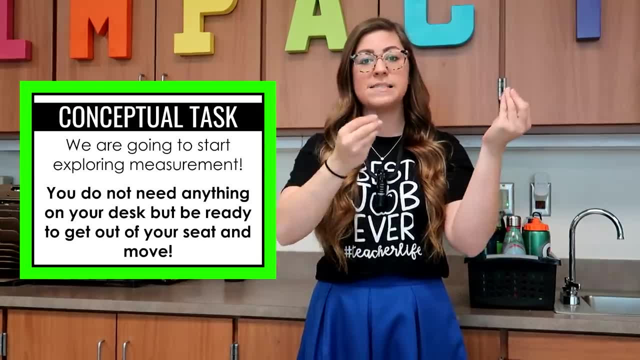 Now just teaching from a math PowerPoint kind of boring, So I like to find ways just to make it a little bit more interesting. So I start off by teaching my students, okay, what is length, What is mass or weight when we get to customer units, and then what is capacity. So we'll discuss what. 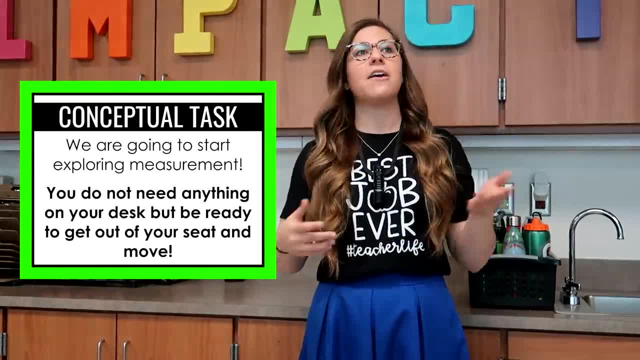 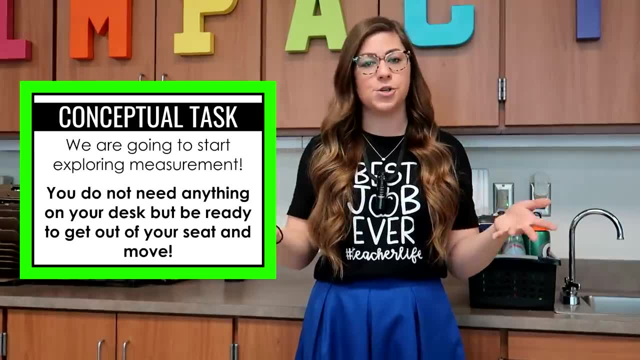 those are, and then we're actually going to practice. So I'll tell them. you know, okay, if you were measuring how much a sandbox can hold which one is, that, Instead of just having them write it down or yell it out, that's not super engaging- I'm going to have them use different. 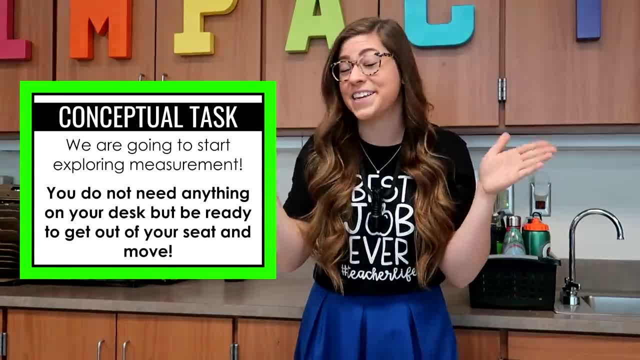 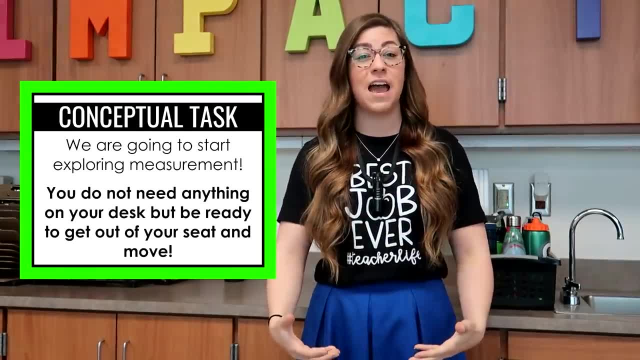 length they're going to go and yes, the sound effect is required. I think sound effects make everything better, So that will represent length. If it is measuring mass, they're going to pretend like they're holding something heavy and, oh you know, kind of grown with it, Like they're. 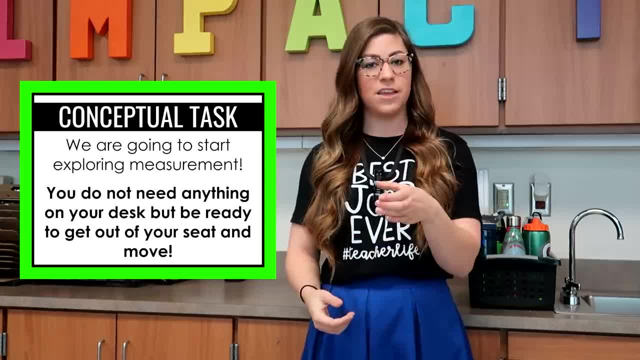 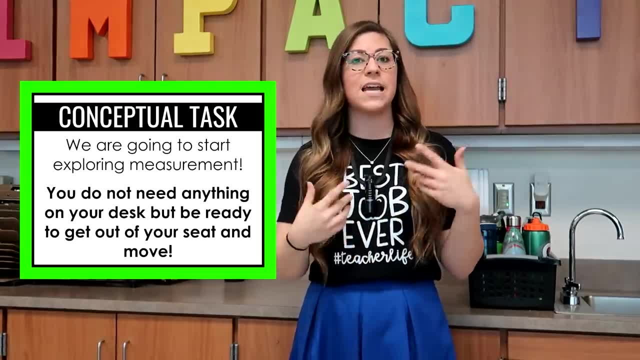 holding something heavy, Then if it's measuring capacity, they're going to pretend like they're holding a cup of water and a pitcher and make a sound as they're pouring it. So we'll do a couple examples and kind of go through which one is which and what kinds of things you would measure with. 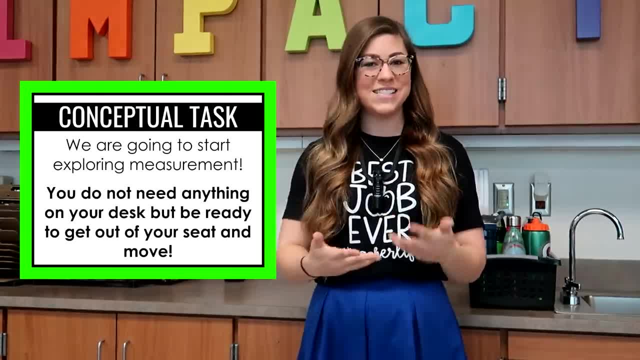 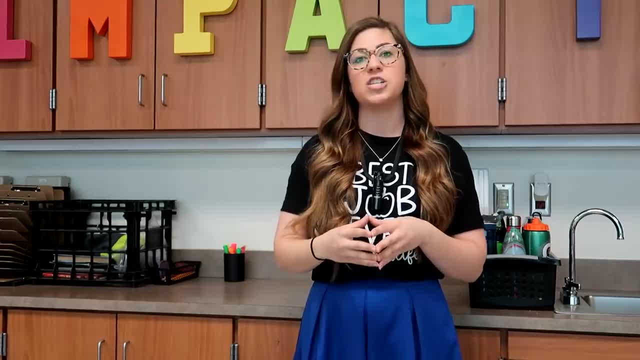 those different types of measurement And they'll do those motions. That way it's a little bit more interactive for them. Then I go through and I actually have them visualize. So we're going to focus on length today, So I want them to visualize how much is a millimeter, how much is a centimeter? 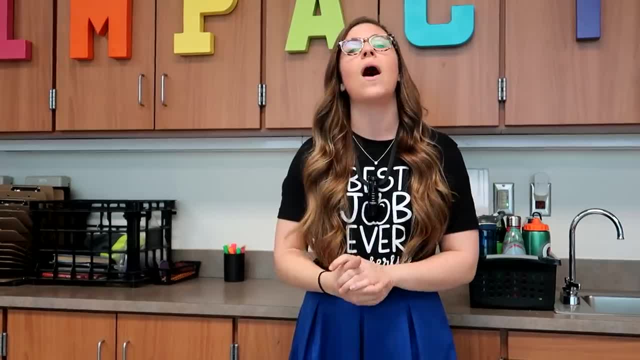 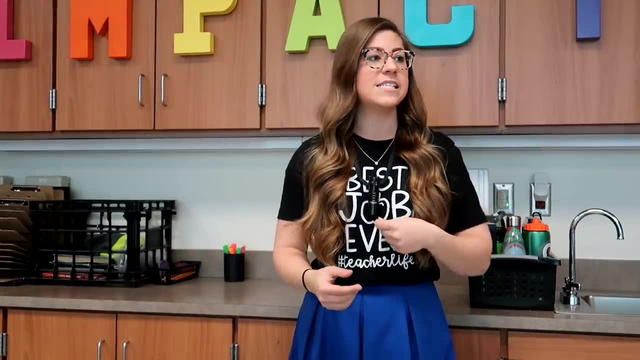 how much is a meter and then how much is a kilometer. So I actually have them close their eyes and I have them visualize. So for a millimeter I usually tell them it's about the length of a grain of sand, And then a centimeter is about the width of your pinky, And then a meter is about the 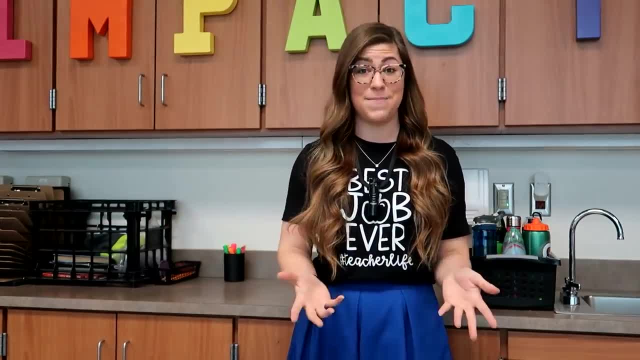 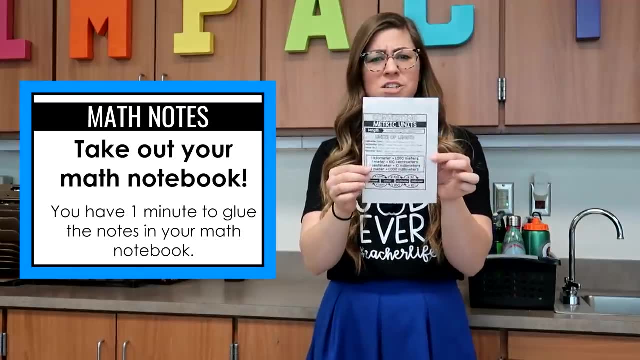 width of a door And then a kilometer is about how long you can walk And then a centimeter is about how long you can walk in 10 minutes. Then I have my students take out their math notebook so I can give them notes. So I create pretty much all of my own notes. Sometimes I do use ones that I can find. 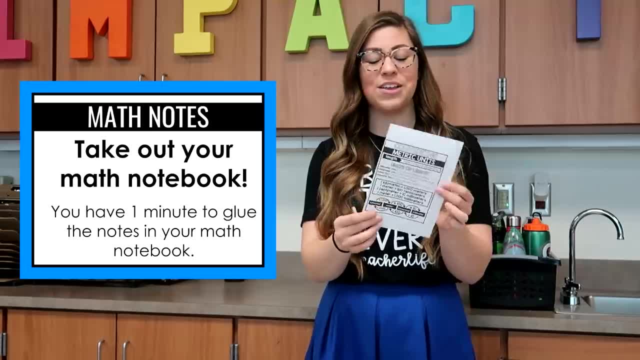 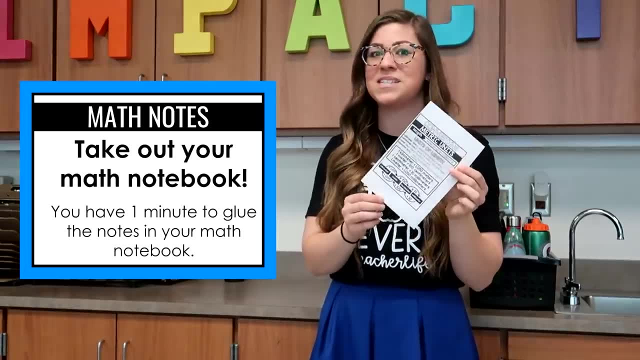 online. I'm sorry I don't have these available yet, but I promise I will. It's kind of my goal for the end of the year is to get up a set of notes. These are not interactive notes- Like the students don't have to copy anything down. but sometimes to save time I just want to give them. 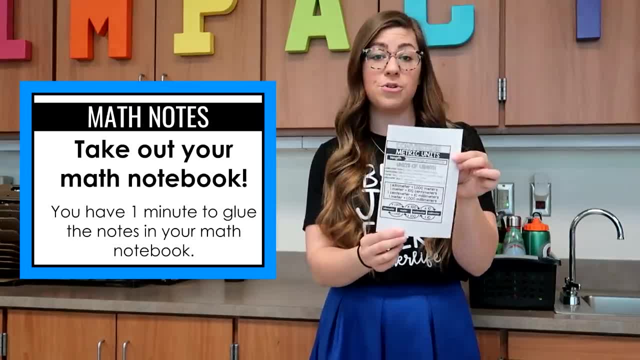 notes that they can refer back to. So I'm going to give them these notes. They will glue them in their math notebooks. Then I'm going to show them a video Now. this video is from number one, number two, number three, number four, number five, number six, number seven, number. 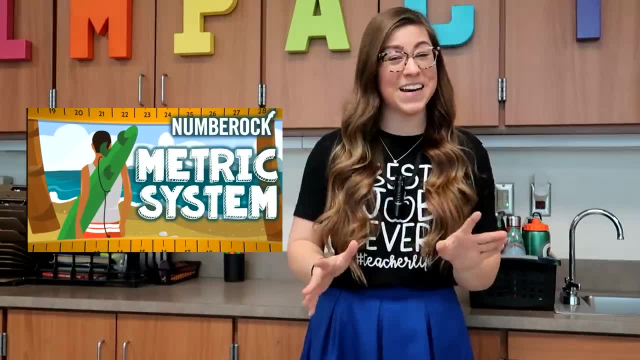 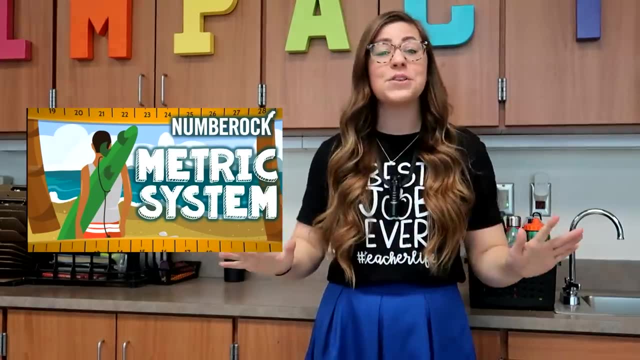 rock And it's all about the metric system. I absolutely love it. It's super catchy. Now it's available on YouTube, So I will leave the YouTube link down in the description box. You can access it for free. It's absolutely just engaging for your students. They really, really enjoy the videos. 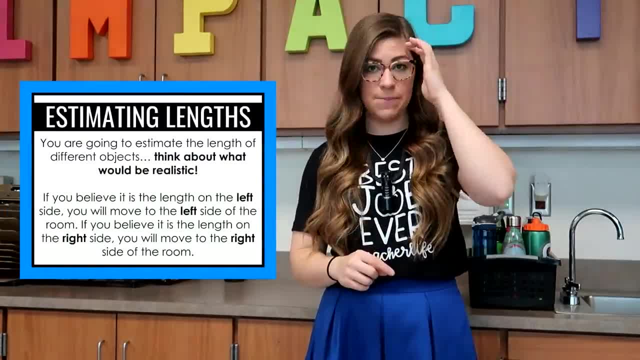 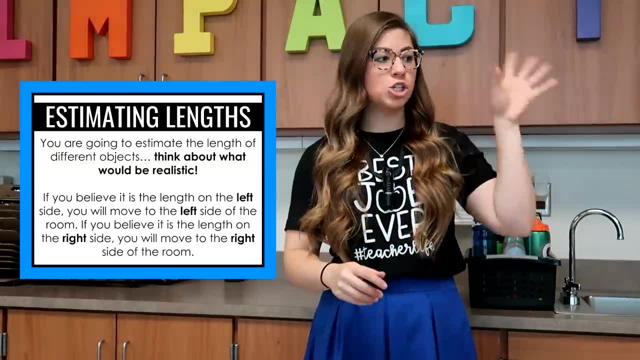 Then I go back to the slideshow and I want my students to practice estimating length so that they can really focus on what would make sense as a length for different objects. So what I'm going to have them do is I'm going to show them different images from the slideshow that I 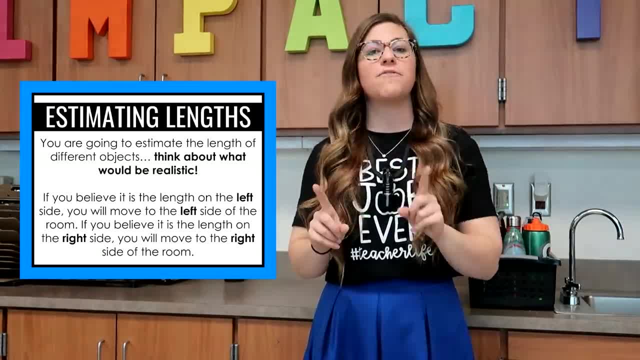 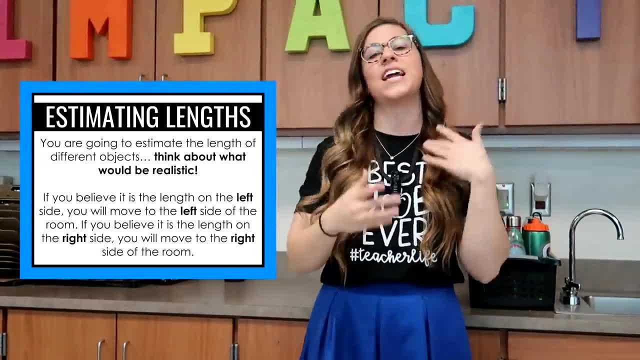 have to choose between two different lengths and which one makes more sense. So if they agree with the length that's on the left side, they will come to the left side of the room. If they think it's the length on the right side, they will walk over to the right side of the room. That way they're. 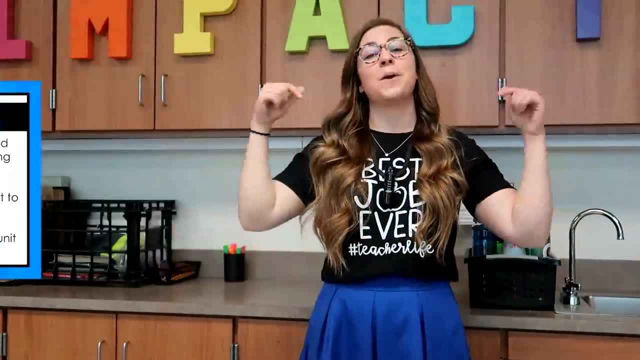 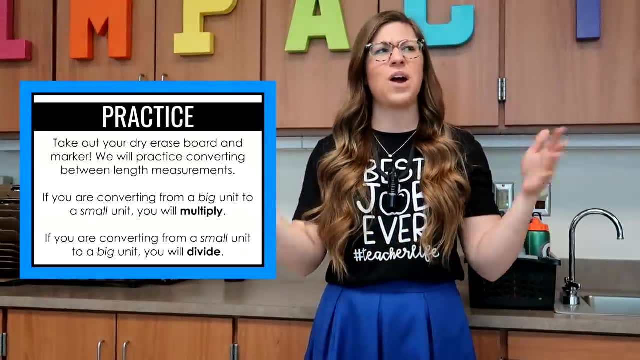 getting out of their seats and they're getting some motion. Then I'm going to have them go back to their seats and we're going to practice on whiteboards. But again, to make it more interactive, I like to tell my students a little rhyme motion, whatever you want to call it, to help them remember. 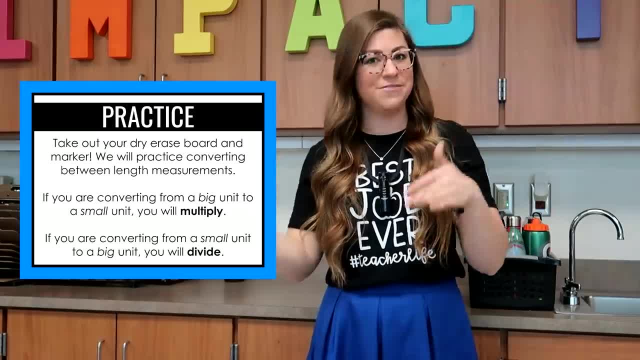 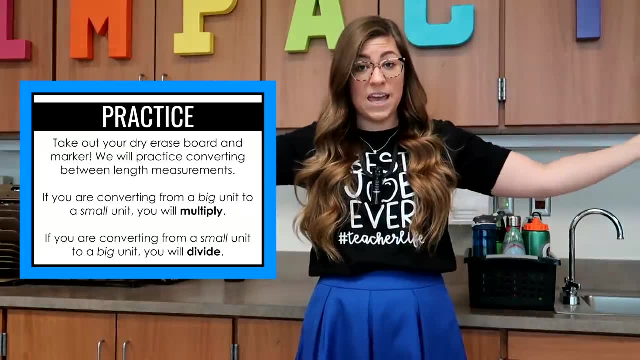 because they always struggle with: do I multiply by 10 or do I divide by 10 or 100 or 1000, whatever it is that they're converting? So I always like to tell my students: okay, if you are going from big, 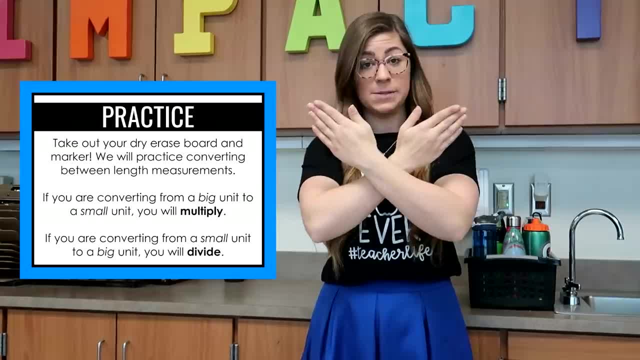 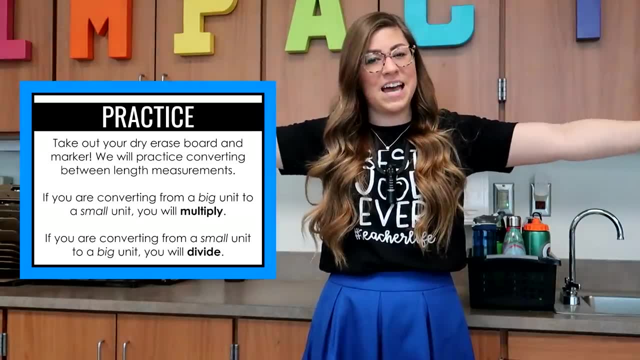 and they put out their hands like this: to small, you multiply. because this makes a cross just like a multiplication sign. Then I tell them if they're going from small to big, they divide, because this kind of makes a division sign, Like if this is the middle line, and then like your head and your feet. 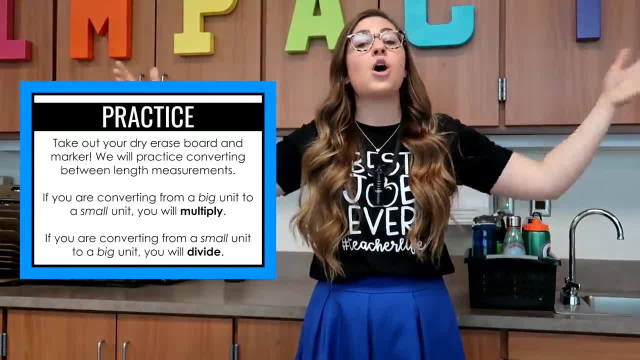 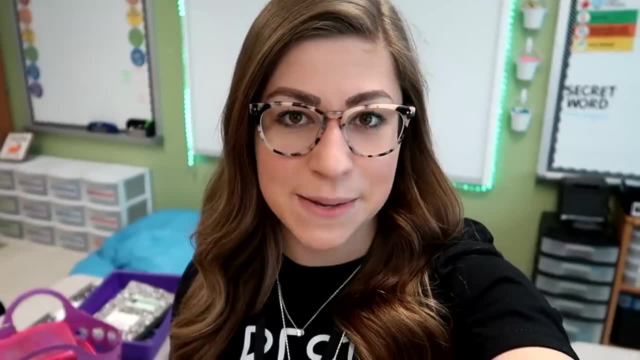 can kind of be the dots. Okay, It doesn't really work, but it works well enough. So as we practice, I have them do that to practice, so they know if they're multiplying or dividing. So hopefully you guys have learned a lot of ways to make lessons more engaging. Now I also sometimes 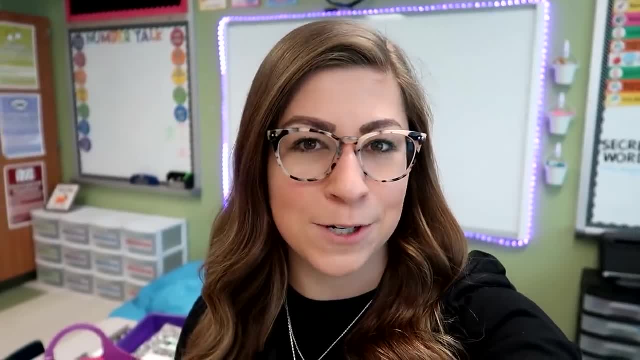 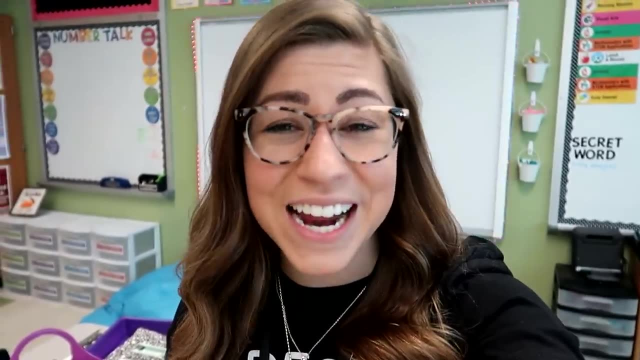 stand on tables and I also sometimes teach in accents. Ultimately, it just comes down to working in opportunities for movement and finding ways for your students to get more engaged in the material. So I hope that that was helpful for you. If not, I'm sorry. And before anyone asked my 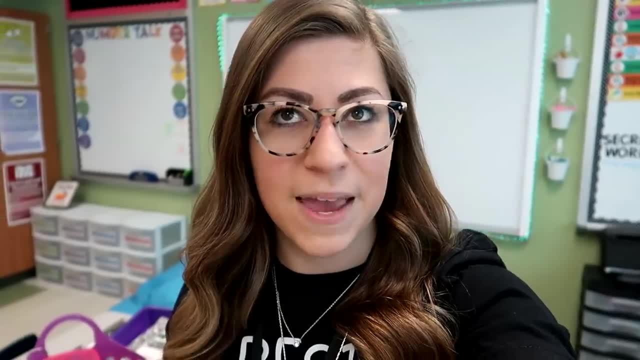 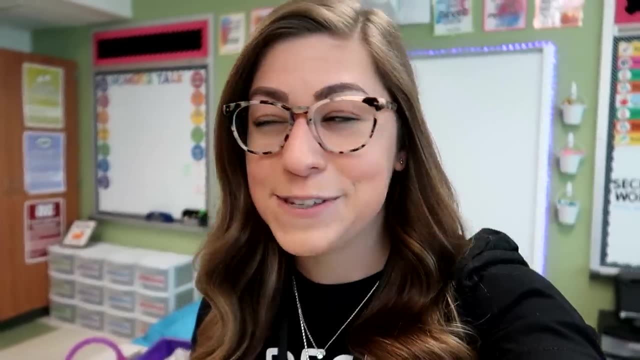 slides like my daily slides. I can't put up the actual slides for sale because they're based on our curriculum. Like I said, I pick and choose, but I do plan on getting a template available. but right now grad school is kind of taking over my life. 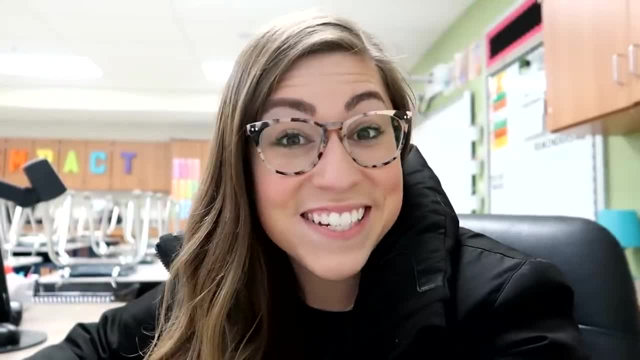 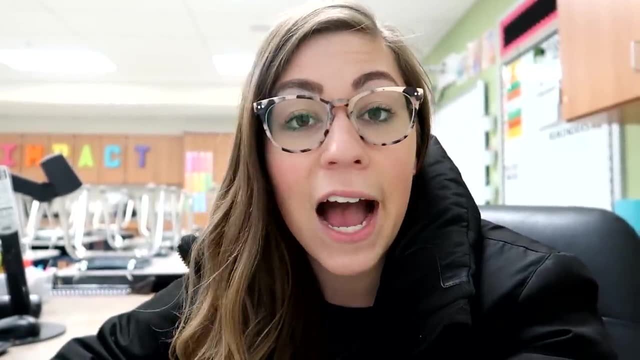 So that will happen eventually, Probably over the summer. So just bear with me. I just took my students out for dismissal and surprisingly, it's four o'clock. I feel like usually by the time I blog it's like six, six, 30,. but I'm going to get out of here early. today I was able to get all my planning done. 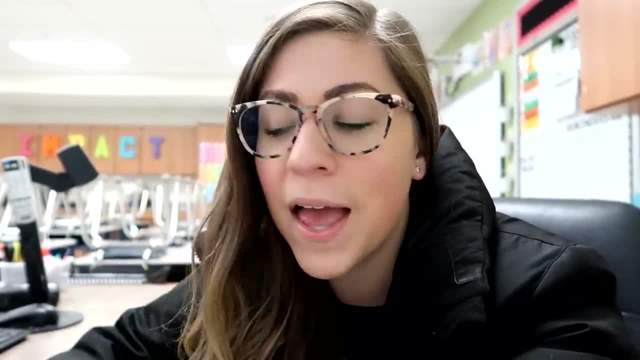 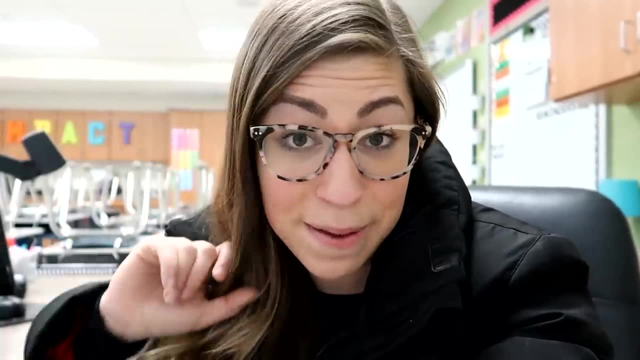 for tomorrow earlier today during my planning time. So that was awesome. And I have been staying late like a lot, which typically I don't mind doing, because what happens is Billy and I go and at the gym after school. So I don't really have a reason to leave early anyway, except for today. So 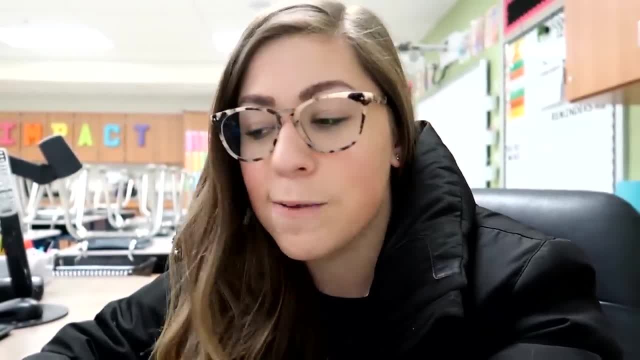 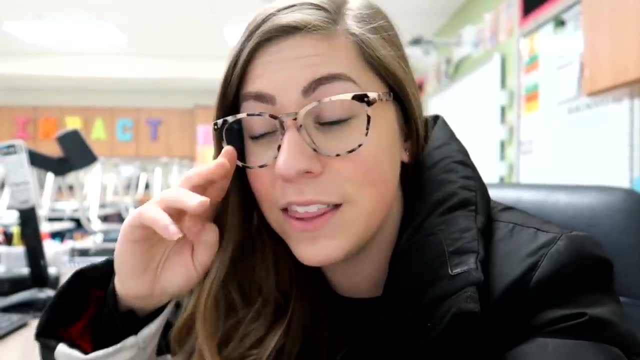 I told you that I did a giveaway of the doorbells on my Instagram, So I need to get to the post office so I can send those off to those two winners. check my PO box And then I think I'm going to go get a haircut- nothing like major, I'm just going to trim the ends. but I have not. 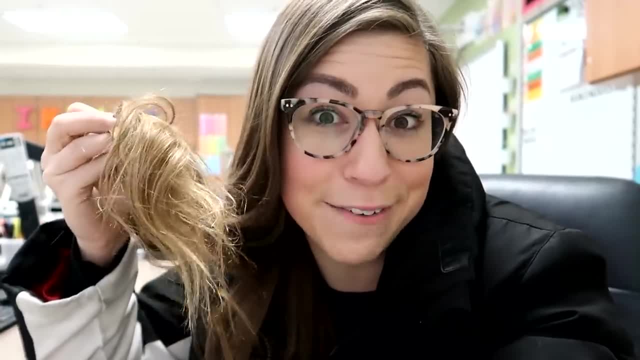 had a haircut in like literally a year. I'm that bad person who never gets their haircut And I get a lot of questions about my hair and like, Oh, what do you do to it? And I'm like I am the worst. 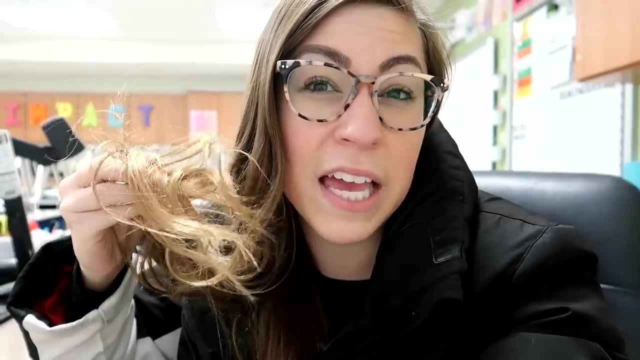 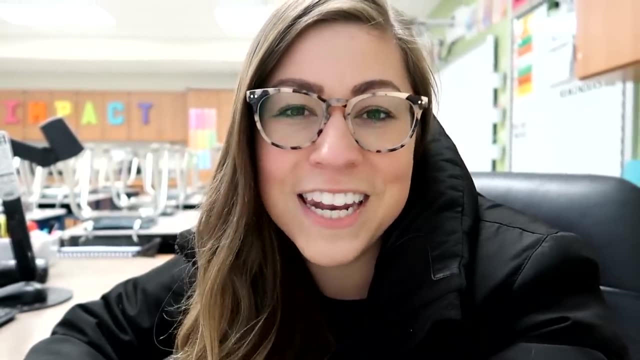 hair maintenance person ever. So I need to go just get all my like dead ends, Like do you see that That's disgusting? I need to go get those all cut off And I will go to the gym and go home and start my next grad school assignment. I will catch up. 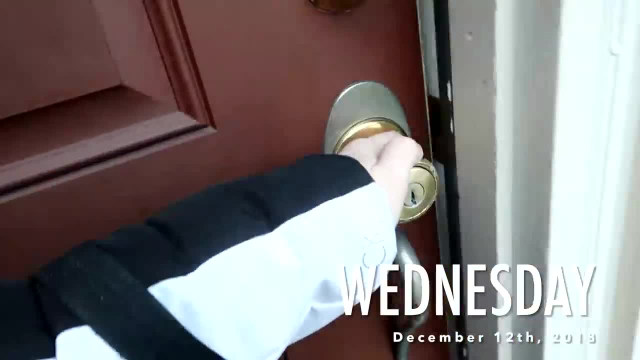 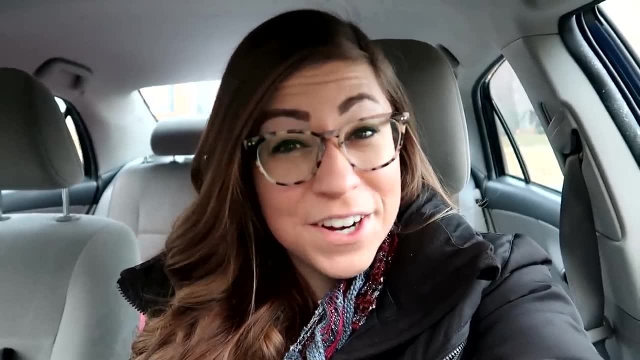 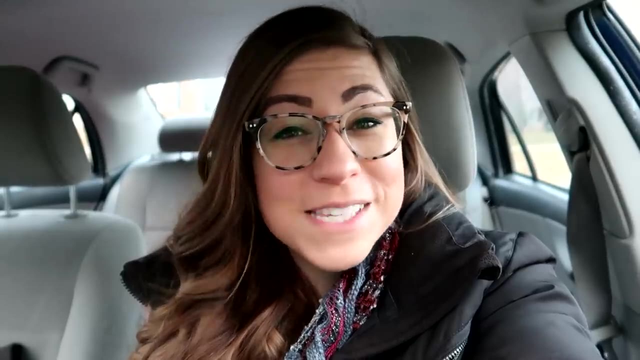 with you in the morning. Good morning YouTube. You know, up until today really I was feeling better. Like after Monday morning I said my throat was hurting, That had kind of gotten better, My stuffy nose had kind of gotten better. And then I woke up this morning and I have a lot of. 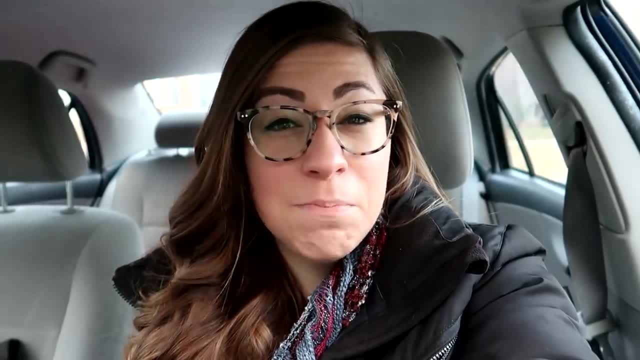 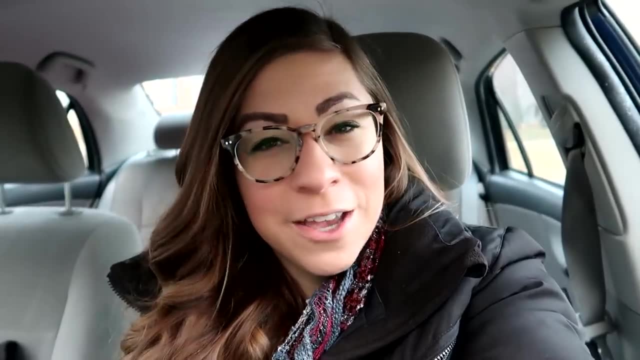 congestion, like in my chest, and my voice has been weird. It's just not good And I'm not happy about it because I was doing better, but it's okay. It could be a lot worse And you know I'm still good enough to like go to school. I do think I'm going to go get. I don't want coffee. 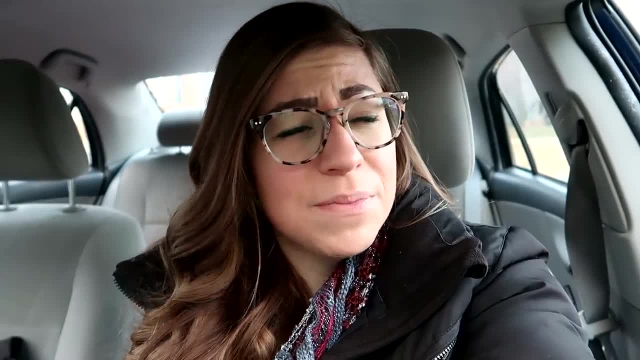 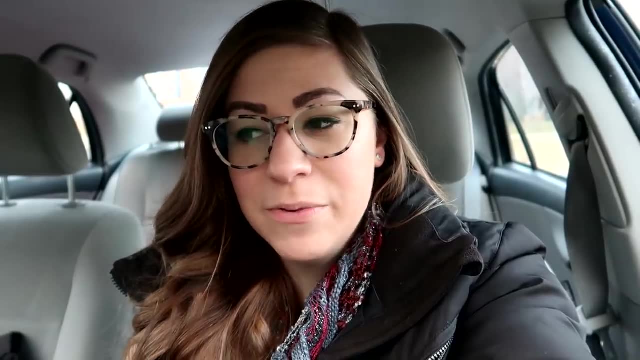 but I want something like cold to drink, like some tea or something like some iced tea. So I'm going to go get that. And then I have a meeting this morning- CDM- And then I have to meet with my team teacher during planning time. 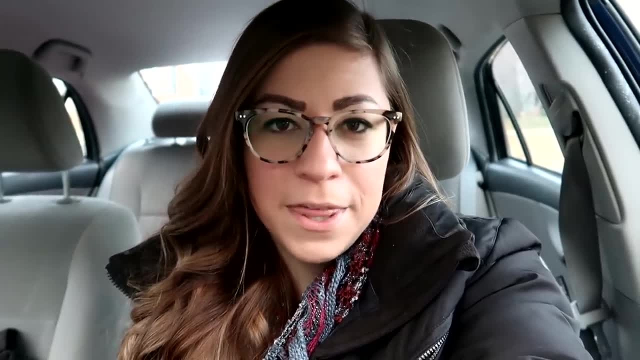 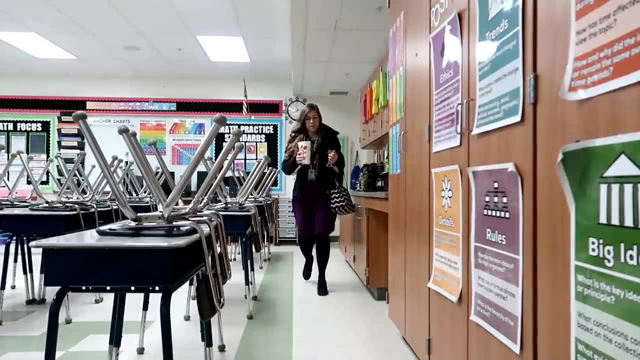 So I probably won't vlog a whole lot today, but you know, I'm here, I'm doing my thing. Look how cute he is Going to work in his suit. It is the end of the day, but I have to make this short because, as you can tell, 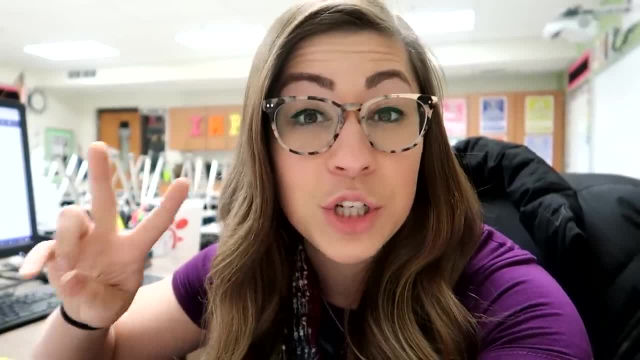 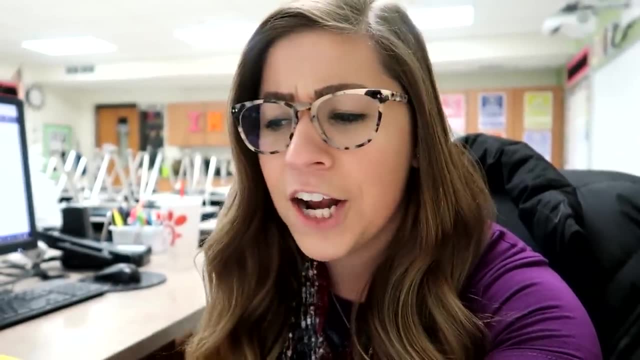 I do not have much of a voice. Now I wanted to share two things that happened from the day. So number one: on the way to lunch I had a student swinging his lunchbox and all of a sudden he goes: wait, I can't swing my lunchbox. I got a Twinkie in there And I just cracked up because it's the 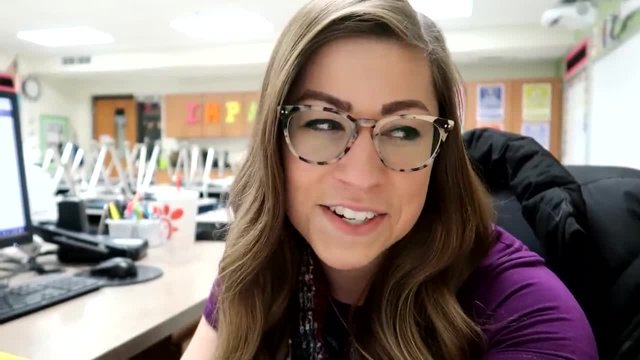 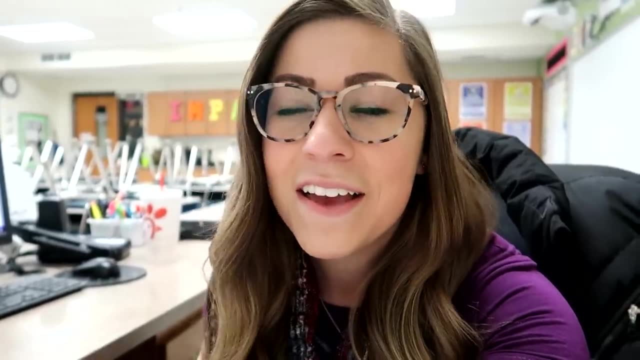 little things like that, You know. it just brings you back to the fact that, like, these are kids. Now the second thing was not necessarily a good thing, but I got hit in the face with a football at recess. It was a. it was a foam one, So it was okay. Like it hurt, but it. 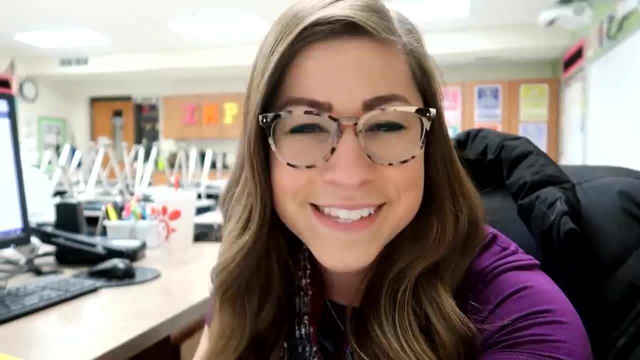 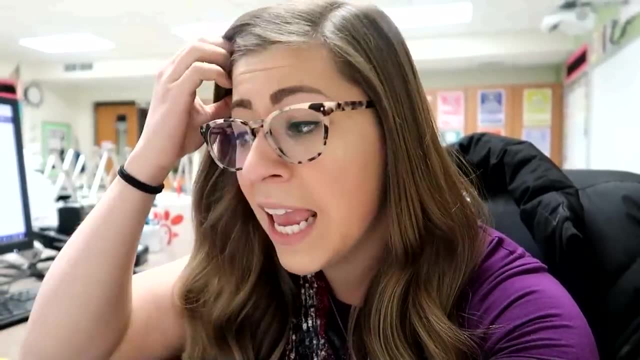 kind of knocked my glasses off, but I survived. It's okay. And it was an accident, No biggie. but you know college does not prepare you for that. I am working on planning out my stuff for tomorrow and I have some fun activities planned, So hopefully I have more of a voice. 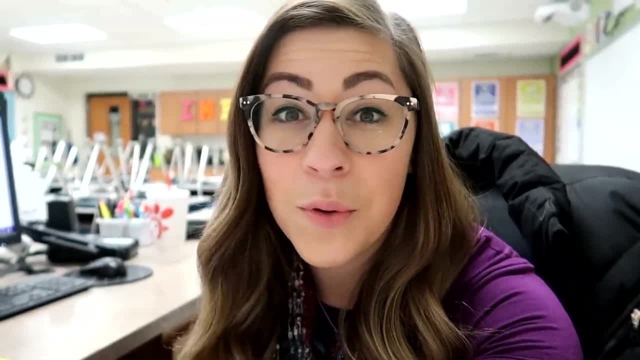 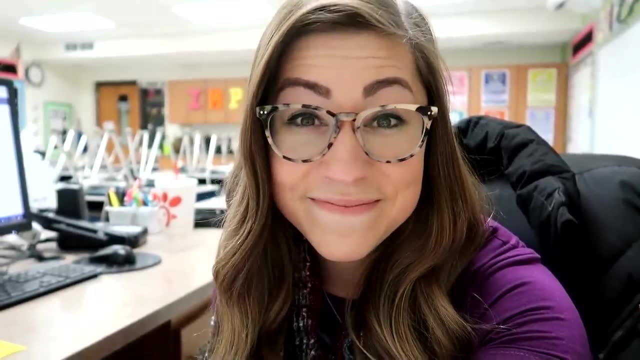 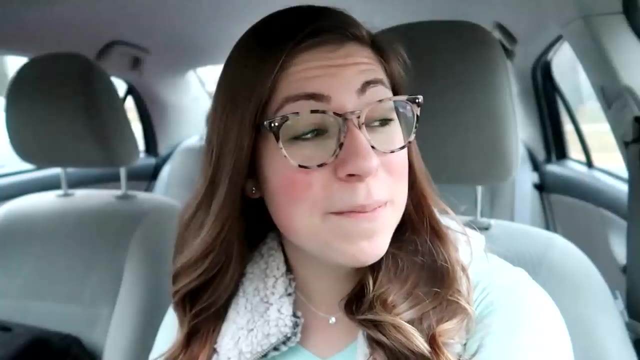 tomorrow and can share those with you. But for now I'm going to just keep my voice off the rest of the day. Try to conserve it for tomorrow and I will catch up with you in the morning. Good morning YouTube. I'm going to keep this short because you know can't talk right now. 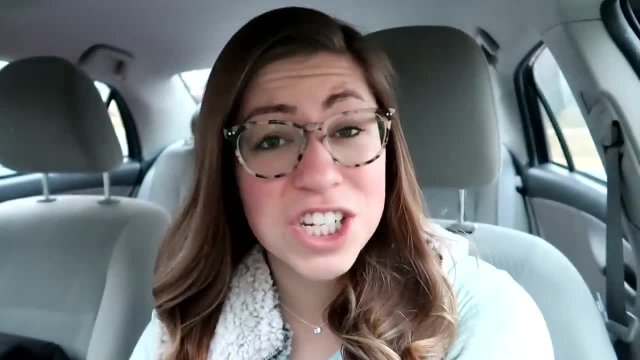 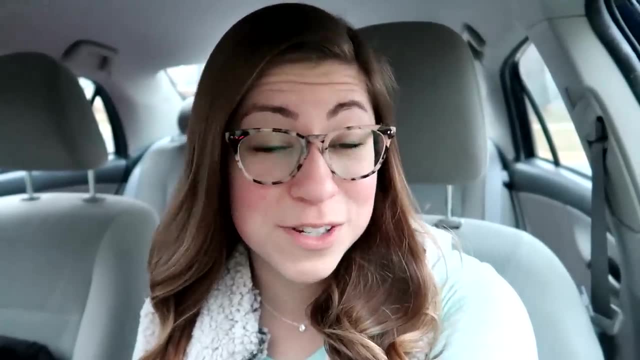 I have SGA committees this morning, So I'm one of the chair people for an SGA committee- that's Student Government Association. So I have a group of students coming to my room this morning before school starts. We are part of the appreciation committee, So 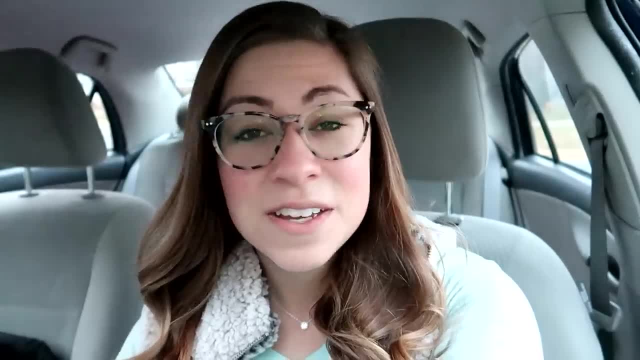 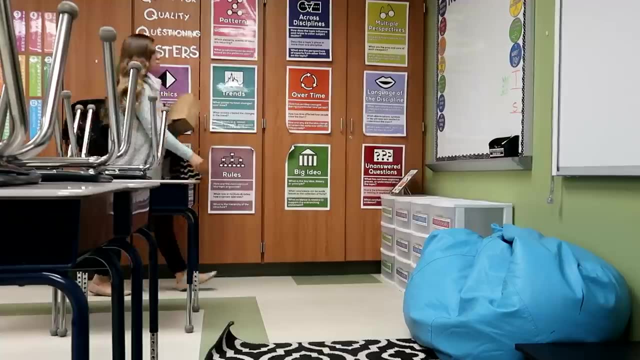 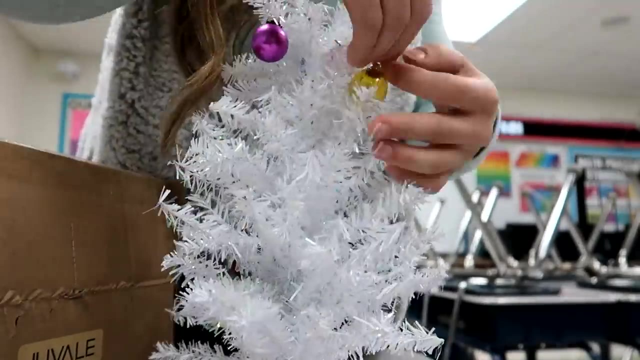 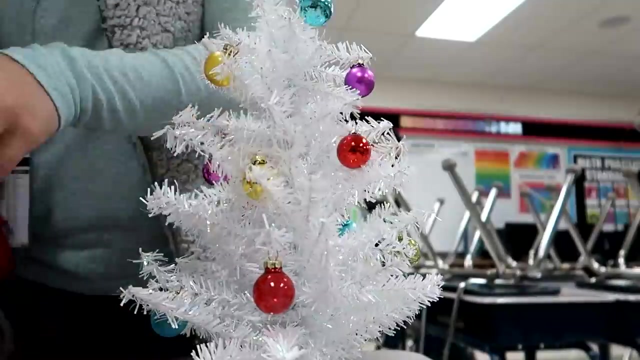 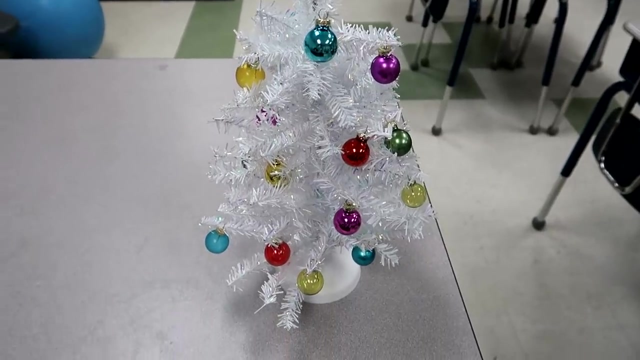 I kind of got it, So I'm going to throw together some stuff for that and just try to survive today. That's what we're doing- We're surviving. So here is the finished product with my tree- Super cute, I know The tree itself came from the Target. 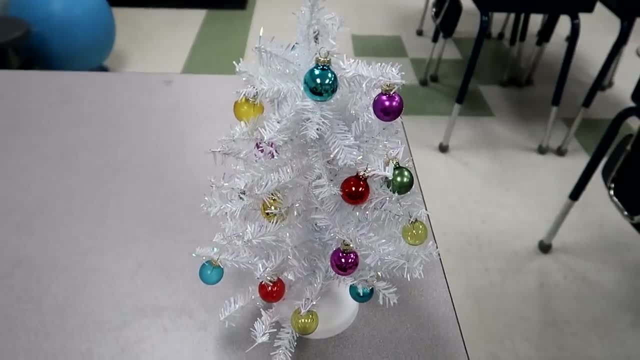 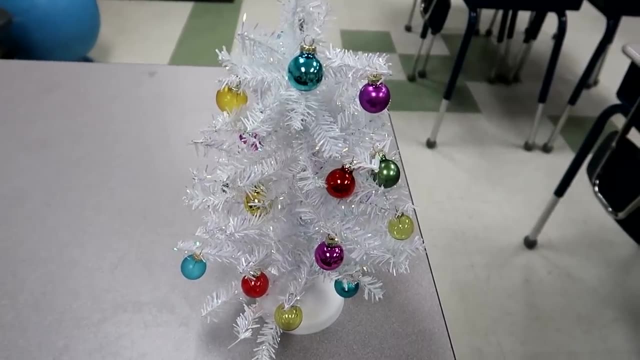 Dollar Spot I want to say it was like $3.. And then I got the mini ornament bulbs off of Amazon and I will link those for you in the description box. And before anyone asks: yes, all of my students do celebrate Christmas. All right, I'm going to do my best to explain this with like. 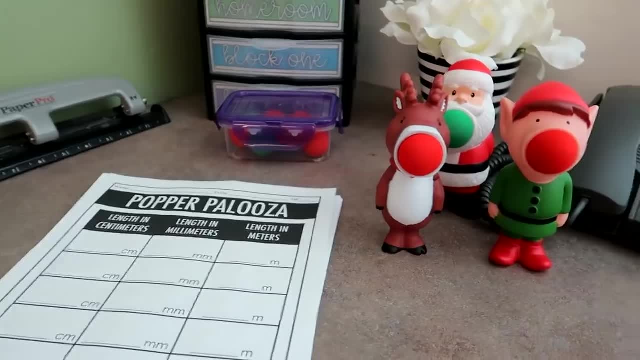 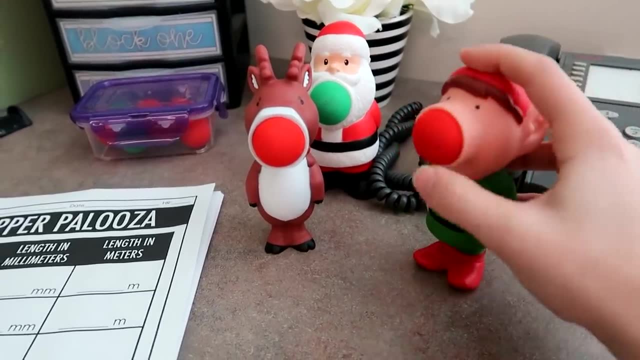 barely any voice. But back in November I had purchased these poppers. So these are from Target. They're like $4 a piece and it comes with the little person and it comes with a total of four balls, So it has the one that's already on them and then 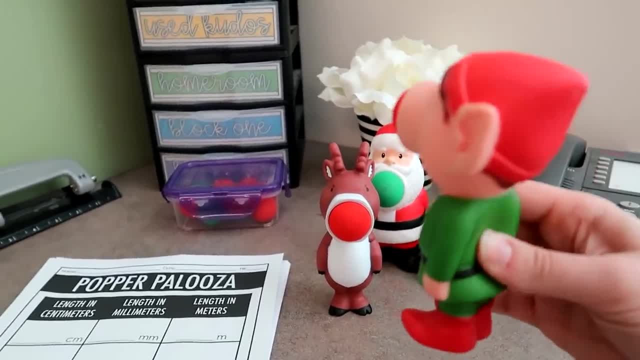 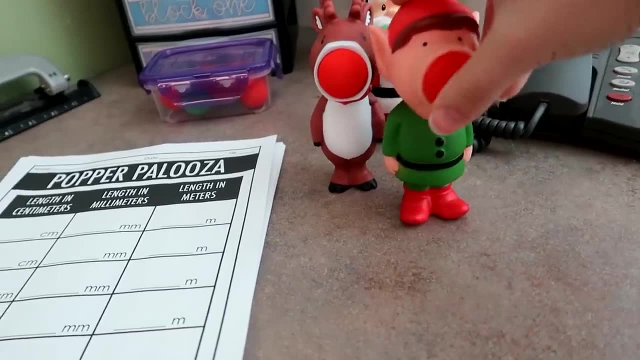 there are three extras. So basically you just squeeze their stomach and it pops it out. So these are super fun. The kids love using them, and I purchased them without really knowing how exactly I was going to use them in the classroom, but I knew that I could come up with something. So 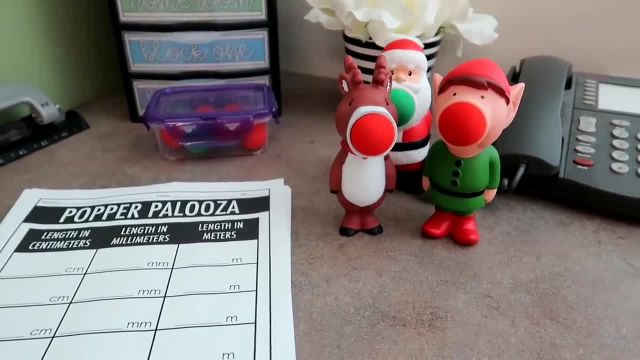 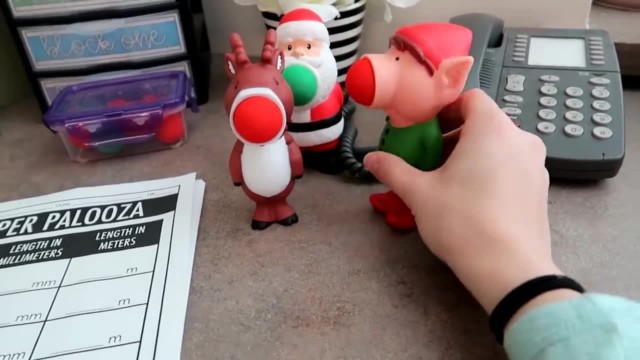 it finally hit me. We are working on metric and customary measurement Currently. right now we're just doing metric measurement conversions, So I'm going to have them work in partners. They're going to pop it as far as they can And I have meter sticks down on the floor. They're going to measure. 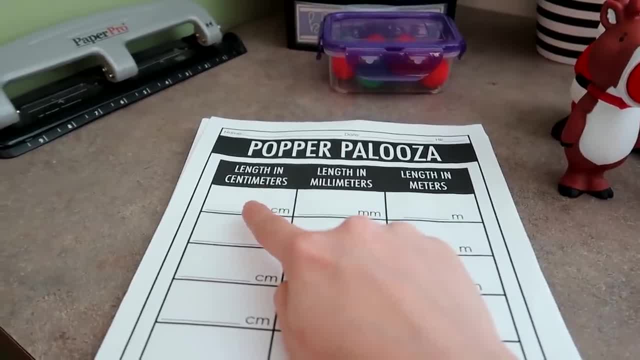 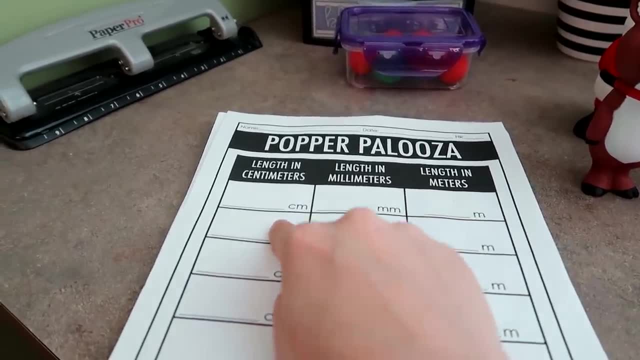 the distance, that they popped it in centimeters, And then they're going to convert that measurement to millimeters and convert it to meters. Now, in order to convert it to meters, they're going to round the length in centimeters to the nearest hundred and then they will convert it to meters. 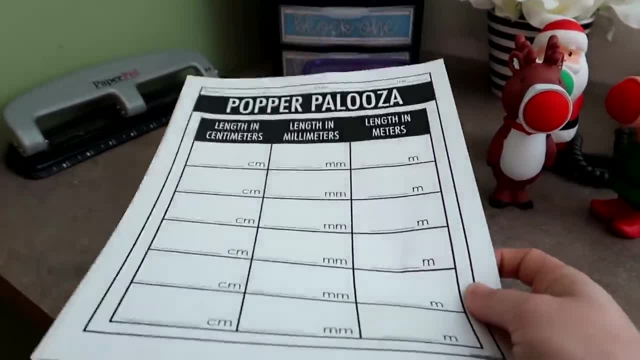 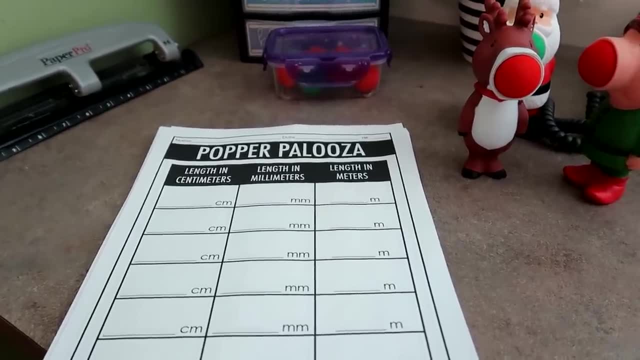 So I just created this super simple recording sheet. If you are interested in this, you can just send me an email and I will send it over to you. I don't have it available on TPT, but If you want it, I can certainly get it to you through email. Didn't really need a whole lot. 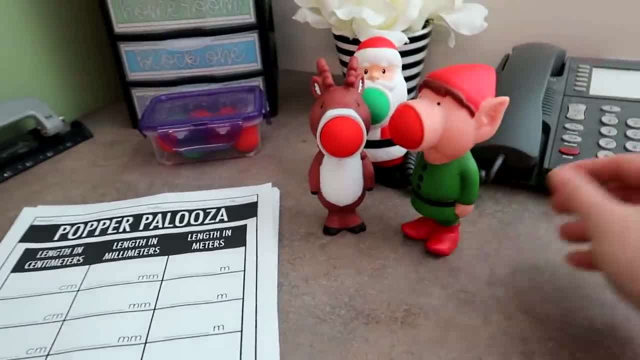 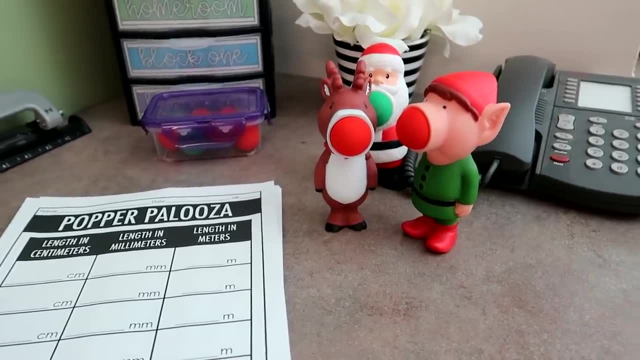 of prep. All I needed were these little poppers and then the recording sheet And what I will probably do after they do the activity today. this could be like an early finisher option later in the week And even next week if they get an opportunity. this is something they could continue. 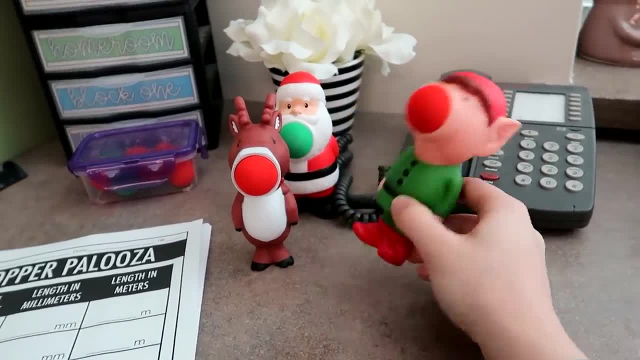 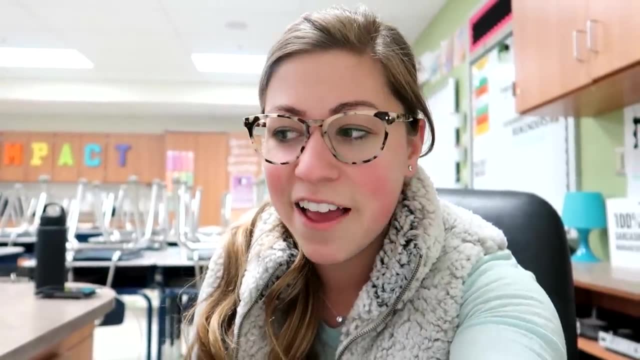 to do So. hopefully, if you have seen these or maybe grabbed them the last time I showed them and you were looking for a way to use them, hopefully this gives you some ideas. So it is going to be a lot of fun. I hope you guys enjoyed this video. If you did, make sure to hit that like. 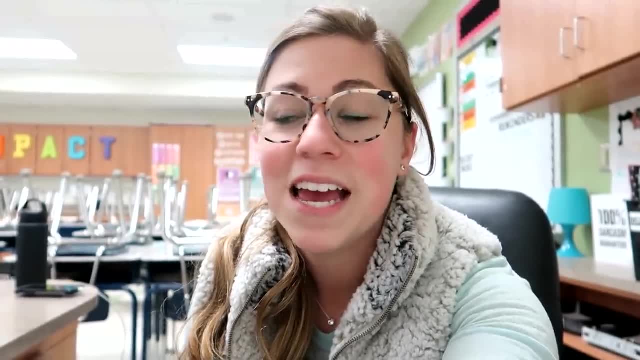 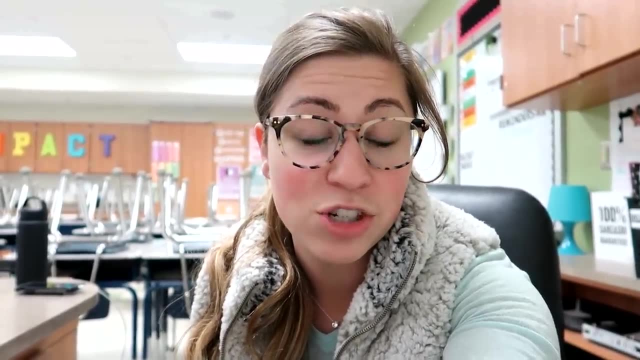 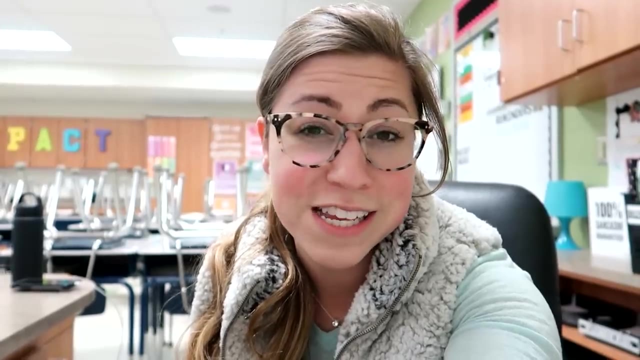 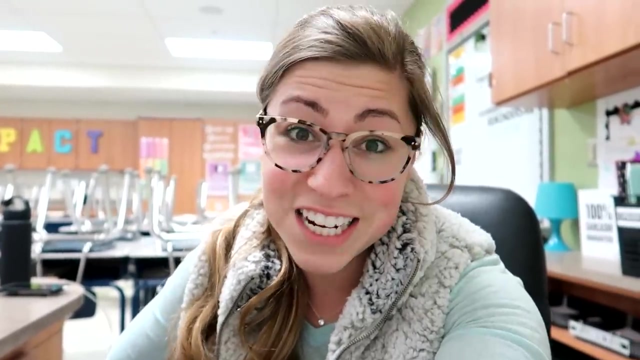 button and subscribe to my channel so you don't miss out on any of my future videos, And I will see you guys in the next video. Bye, I'm just worrying about doing other things and I want to be able to see them play. 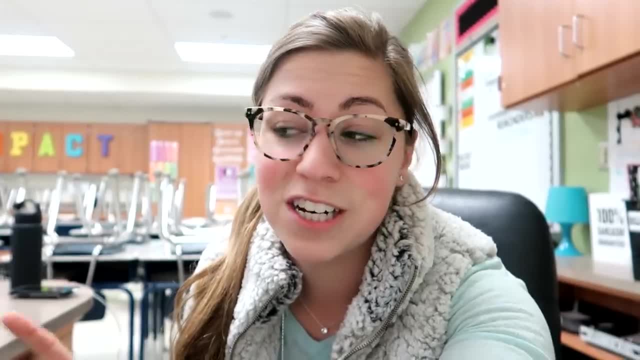 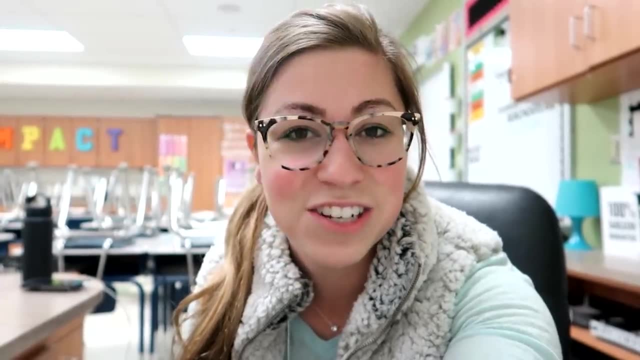 And a lot of my students are in band or strings, plus a lot of my students from last year. So I'm going to be a good person, go to that, Then I will go home. Thankfully, I don't have to do any lesson planning tonight and I can actually relax and hopefully start. 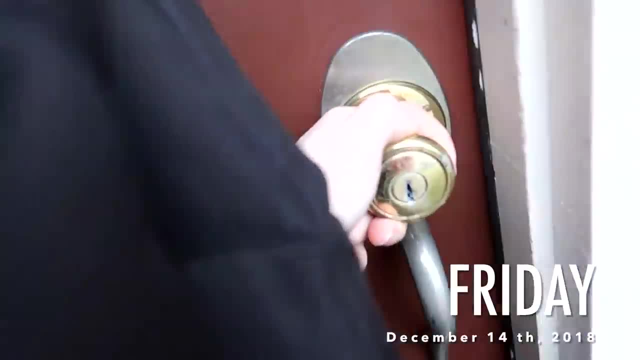 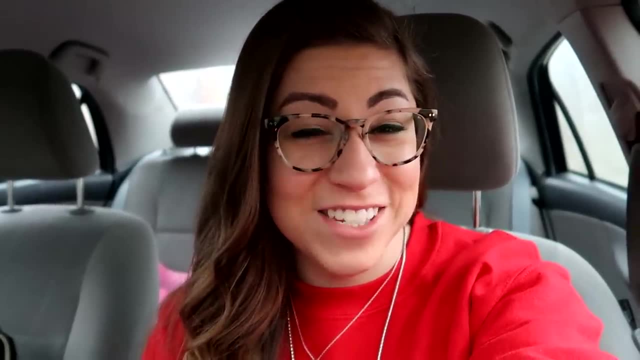 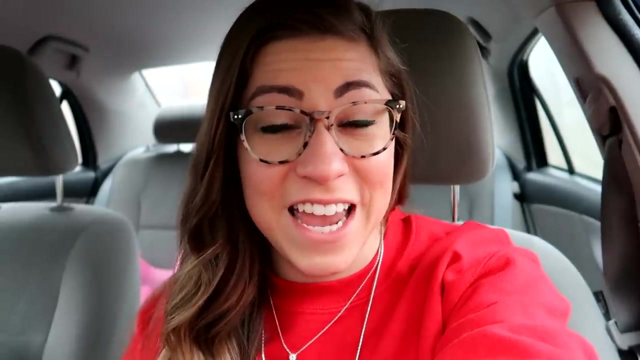 feeling better. Morning YouTube: I feel a little bit better. I mean, I thought my voice was back, but now that I'm actually talking, apparently it's not. The worst part right now is just the, the congestion in my chest and the cough. But good news is, today I do have Chromebooks, So I 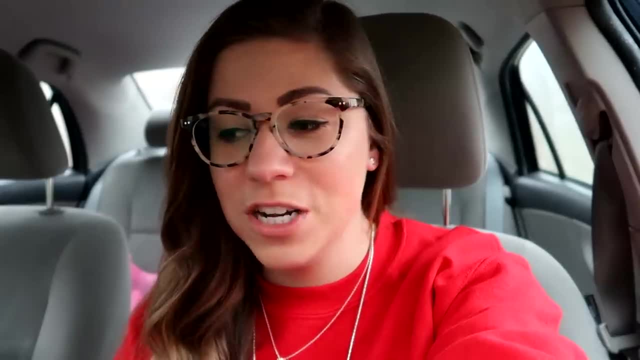 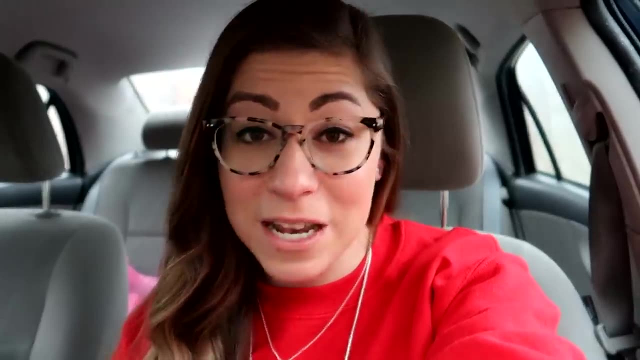 think that that will help and I won't have to do quite as much talking. We're going to do a kahoot and one of my blocks earned some kind of like free time on the Chromebook, So I'm going to reward them with that. I have committee meetings this morning and then I have no planning time, So 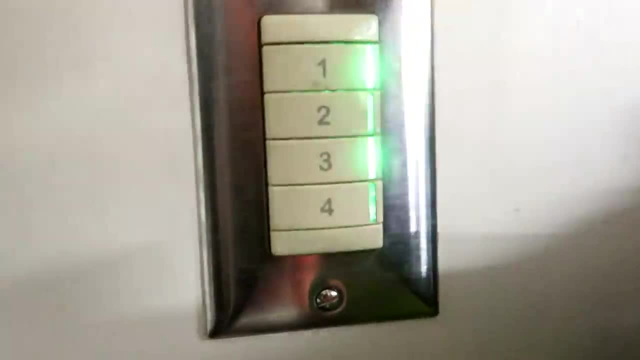 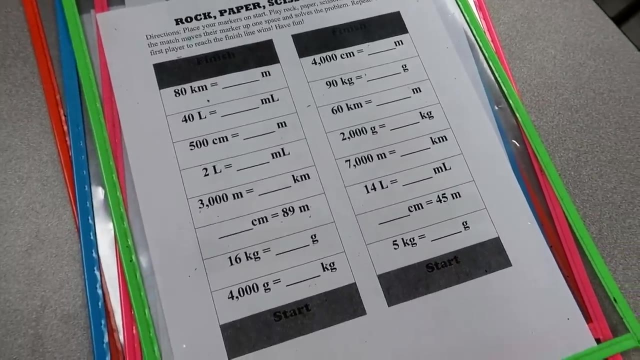 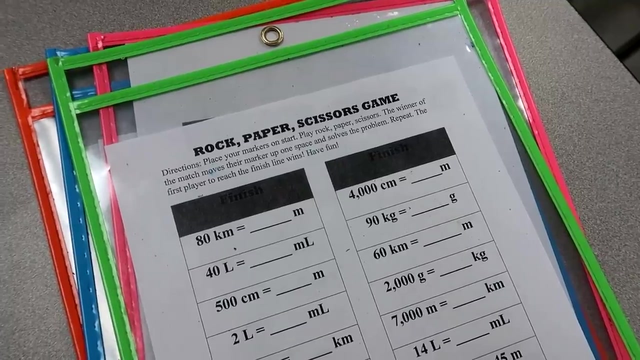 it should be interesting today. I wanted to talk you through one other activity My students. I actually did this yesterday, but I forgot to kind of explain it to you all, So this is called rock paper scissors game. Now, I did not create this. 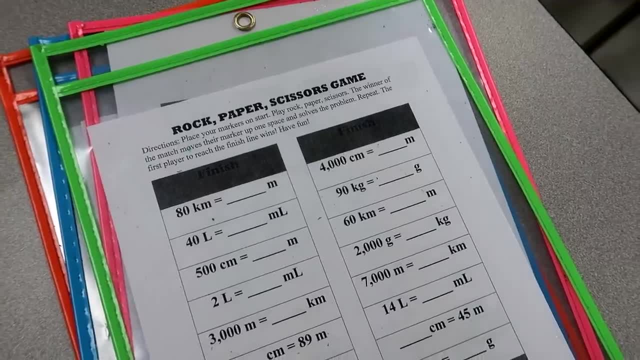 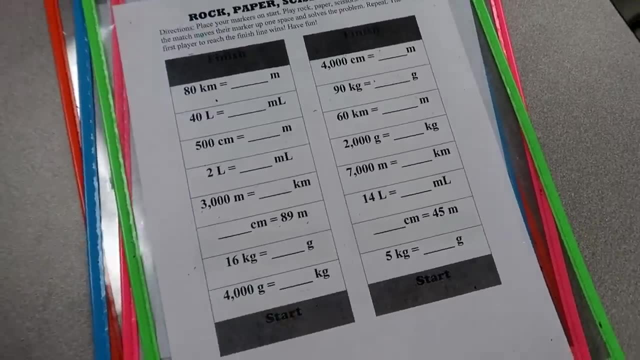 This was something that was given to me, but you could totally take this idea and adapt it to your own classroom. Basically, there are two different sides- is who students play in partners. I'm sorry. I'm doing the best I can with my voice, y'all. 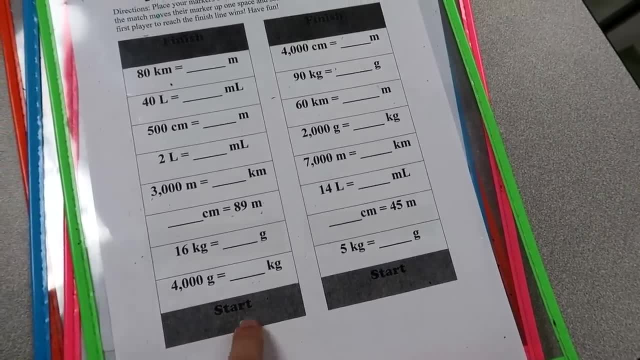 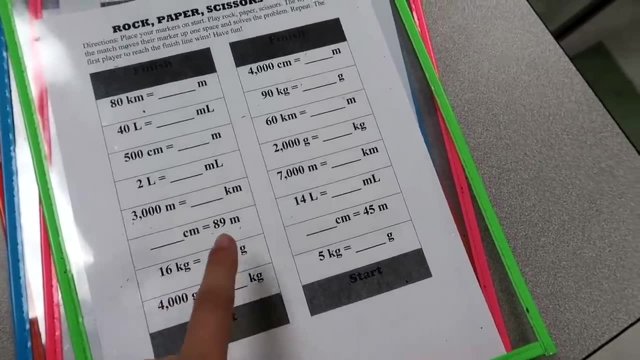 So they start down here. at the start they play rock paper scissors and the winner gets to move their marker up to the next level And they have to solve that problem. And in order to keep it there, then they do rock. 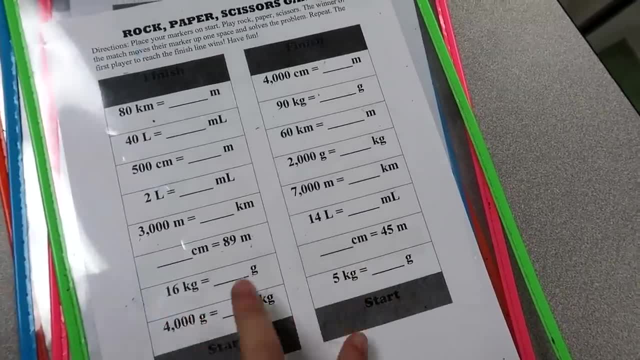 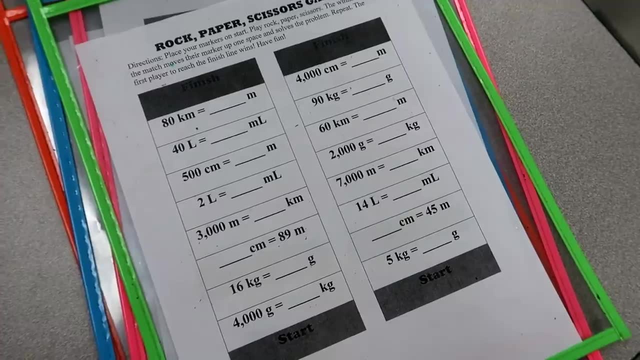 paper scissors. again. let's say, this person moves, they move up to the next level, So it's a race to get up to the finish line. But what I love about this is you could so easily adapt this to any content area or even any grade level. 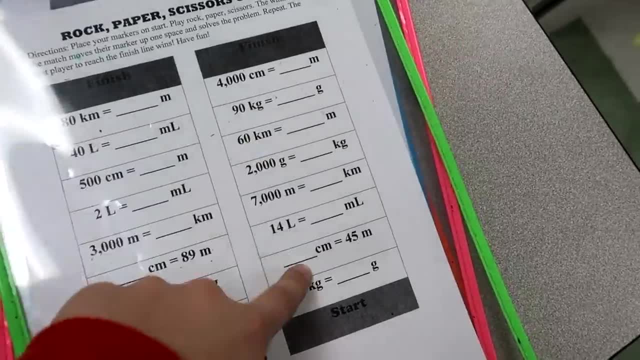 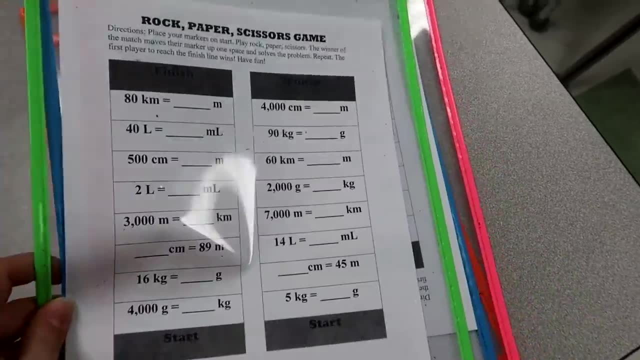 All you would have to do is adjust what is actually in the bars here. So this is just a quick, easy idea. I basically just printed them out, put them in page protector so they could be used again and again, And then this is something you could even have as like an early finisher option. 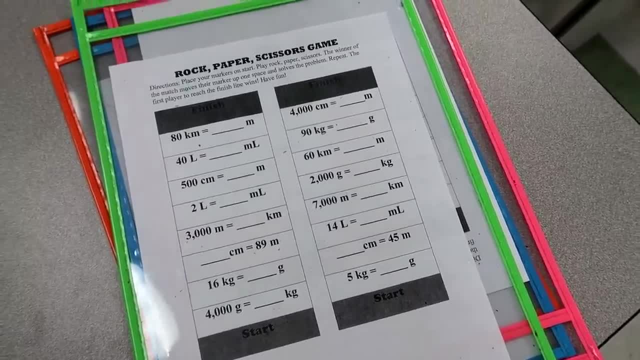 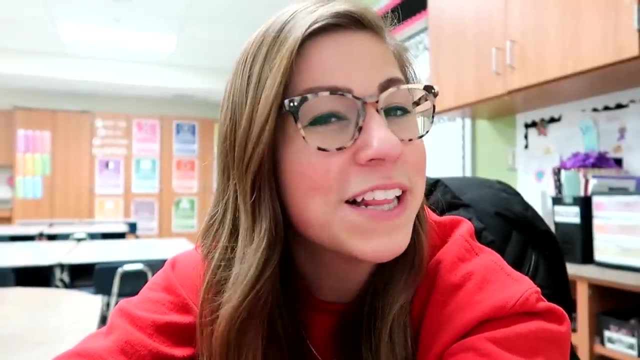 Once you're as students do it the one time, and partners and they understand how to play it could be something that they could always go back to. It is now the end of the day, which means I've survived another week and I am another week closer to winter. 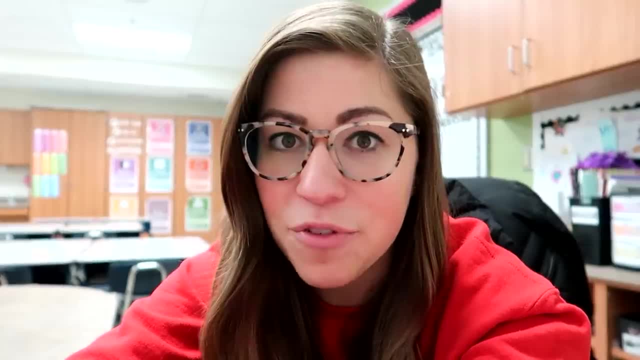 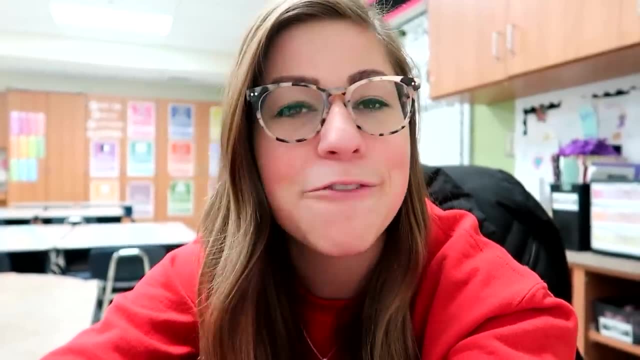 break. We do go through next Friday, so I will have a vlog next week. It'll focus more on kind of like what we're doing for our holiday party and some fun activities and all that good stuff. But it is time for me to end this blog so I can get out of here and go home and 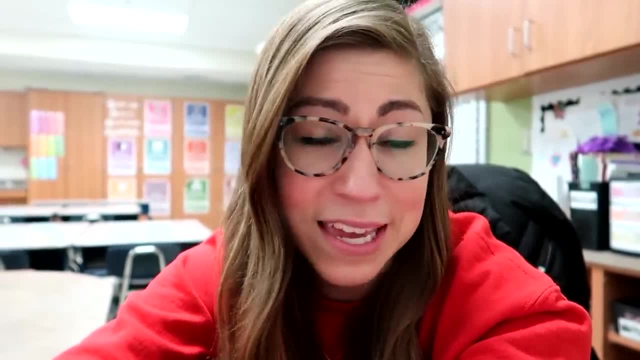 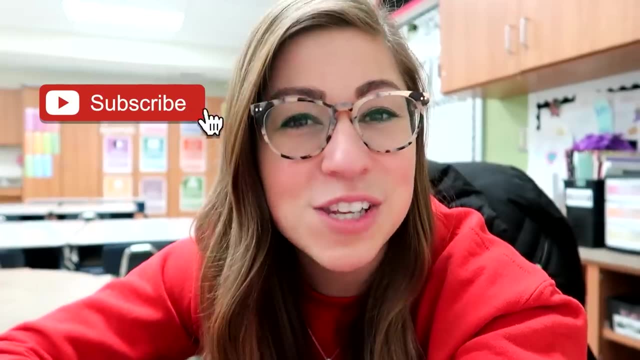 take care of me with not feeling well, Like I definitely need just a weekend to be able to to rest and rejuvenate. so if you enjoyed this vlog, please go ahead and give the video a thumbs up. also, don't forget to hit the subscribe button and the notification bell so you are notified every. 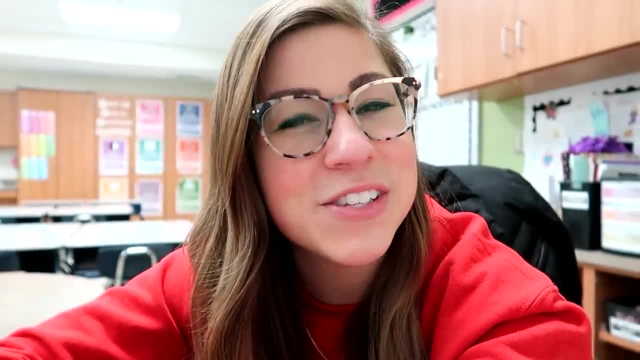 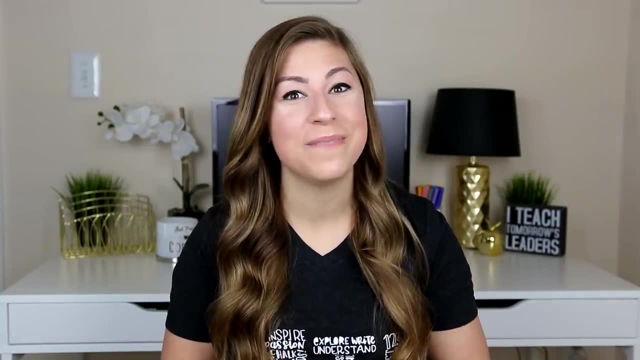 time I post a new video. as always, thank you for watching. I love you all so much. don't forget to think positive and I will catch you all in the next one. thank you so much for watching all the way to the end of this video and for supporting my youtube channel if you want to check out any. 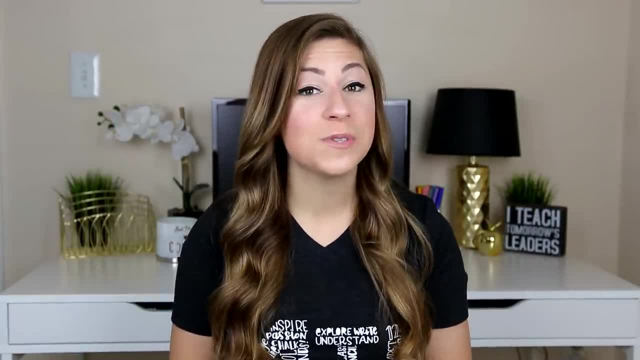 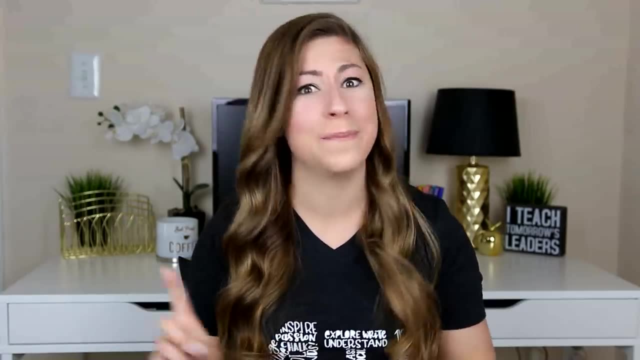 of my older videos. you can use the two links right down here if you want to subscribe to my channel so you don't miss any future videos. you can use the link right up here. the links to all of my social media sites: my teachers pay teacher store, my merchandise store, my amazon store. are in the description box and I'll catch you guys in the next one.